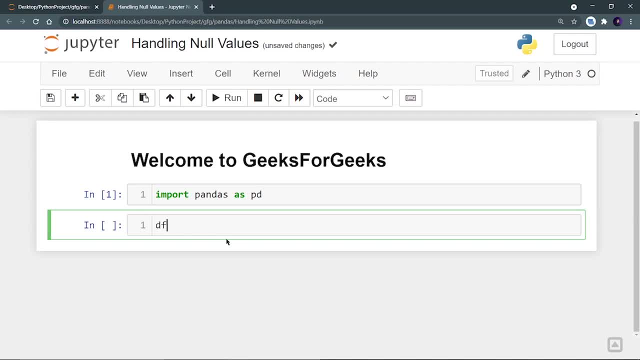 house prices dataset. So first of all, let's create a data frame called df is equal to pdreadcsv- bangalorecsv, And you can download this CSV file from the link in the description. Now let's see the first five rows of this data frame, So dfhead. 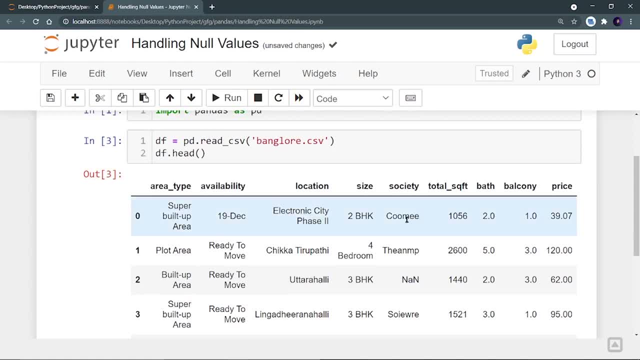 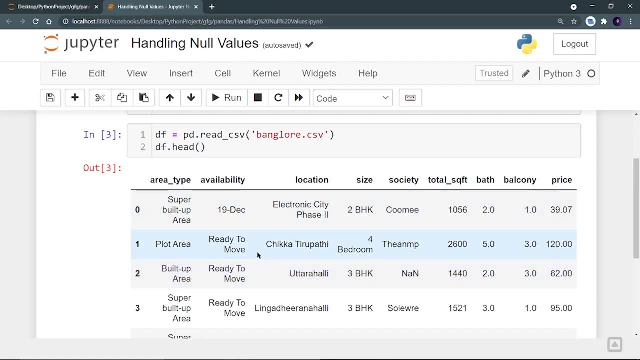 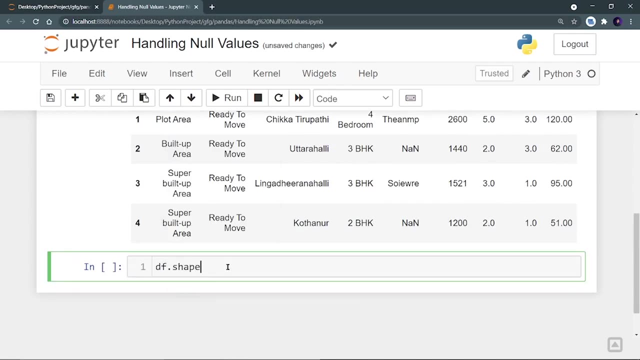 Let's run it And I can see the columns, the features of this dataset, And let's say we have to analyze this complete dataset. So for that, first of all, we need to check what is the shape of this dataset. We can do dfshape, So this is going to return me a tuple which will tell the rows comma. 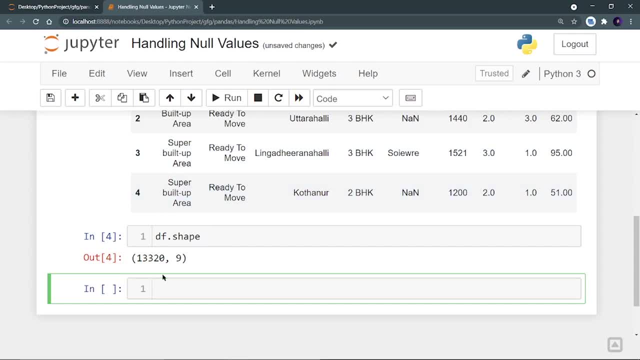 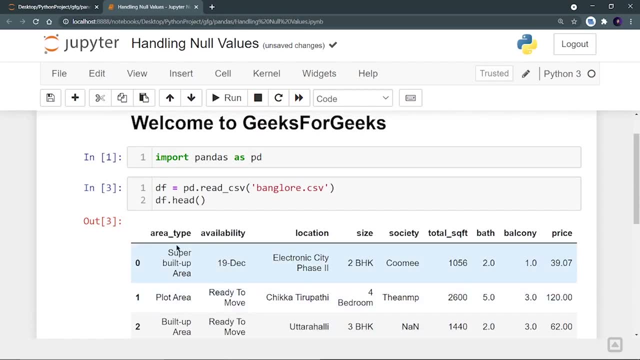 columns. So this means that this complete CSV file contains 13,320 rows and nine columns, And you can also see that 1,, 2,, 3,, 4,, 5,, 6,, 7,, 8, and 9 columns are there right Now. 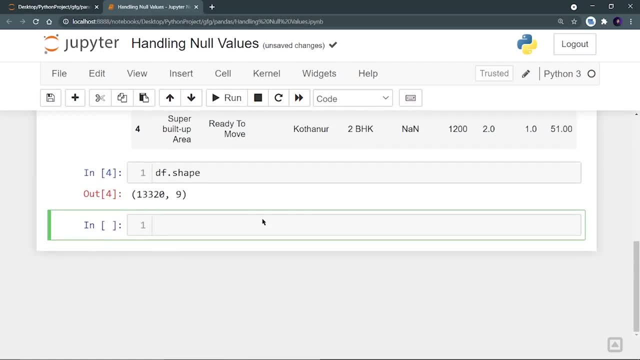 this dataset may contain some null value, right, So we have to analyze it. So for that there is a function called dfisNull. This function is going to return me to, or false, So it returns basically the Boolean value. So, wherever in 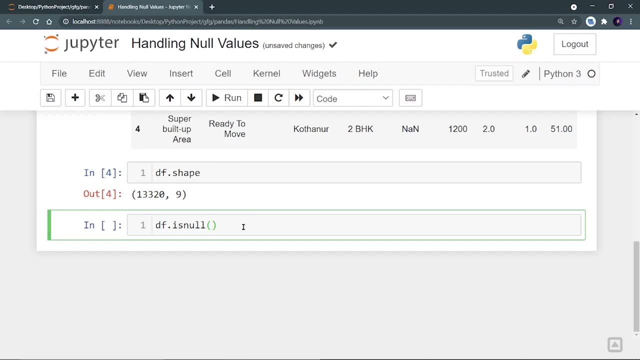 this data set, the null value will be there, then it will be true, Either it will be false, right? So let's run it. So I can see that mostly it is false, but I can see some places. at some places it is. 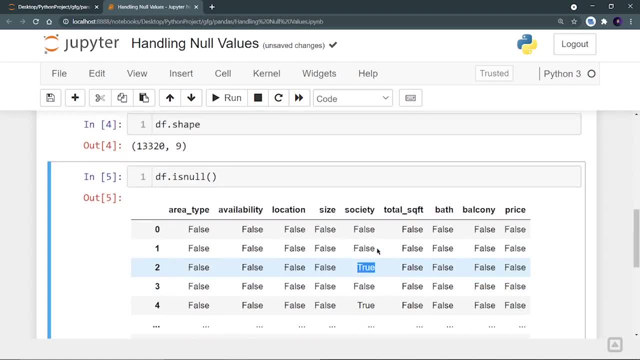 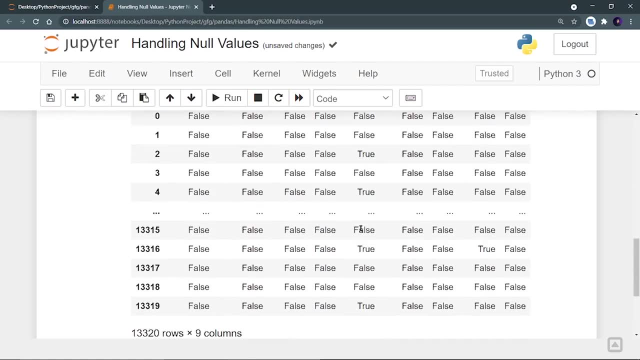 true. So this true means the value at the cell is null, right? You can also see over here: it is NN. NN means null right. Now, I don't want this complete true-false too false. This you are welcome to look into. 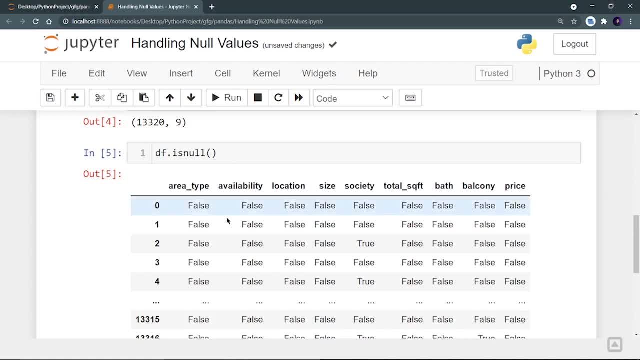 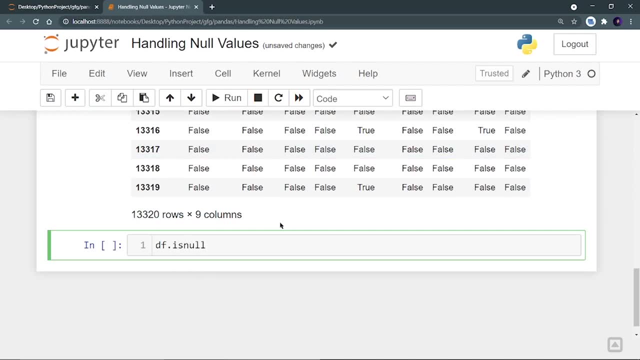 So the value on this cell is always true. And then you have to make sure, do ffAlter. which false thing. I want a total number right For every column. So for that thing, what you have to do is you have to run a function called dfisNullSum, and let's run it So. 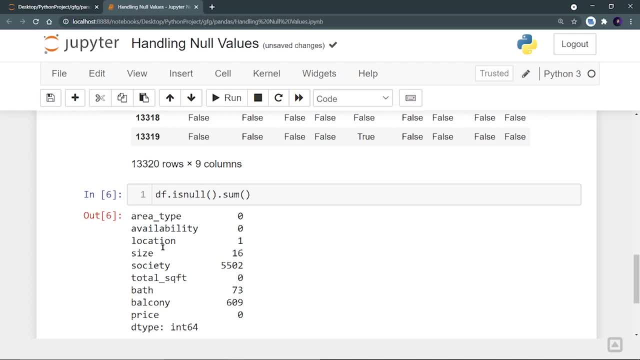 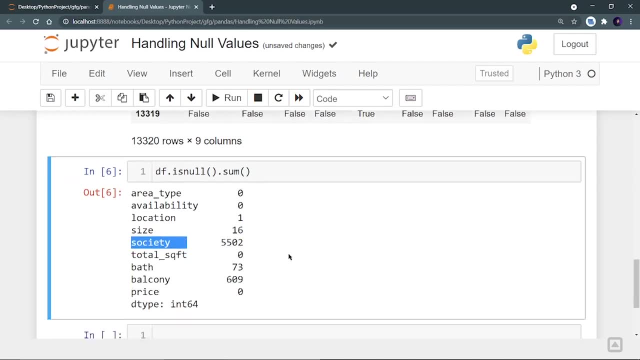 column wise. it is giving me that area type column contains zero null values, location contains one null value, size contains 16 null values and society column contains 5,502 null values. right, So this gives me the total sum of the null values in each column. Now, 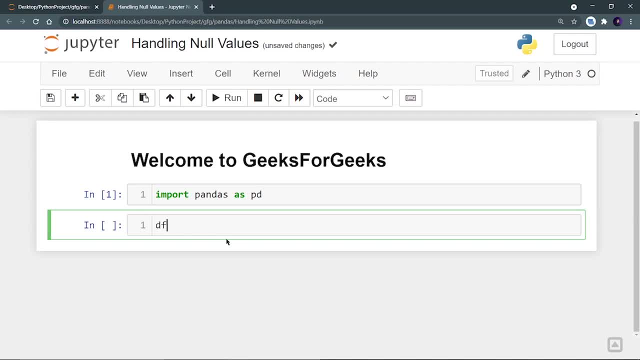 house prices dataset. So first of all, let's create a data frame called df is equal to pdreadcsv- bangalorecsv, And you can download this CSV file from the link in the description. Now let's see the first five rows of this data frame, So dfhead. 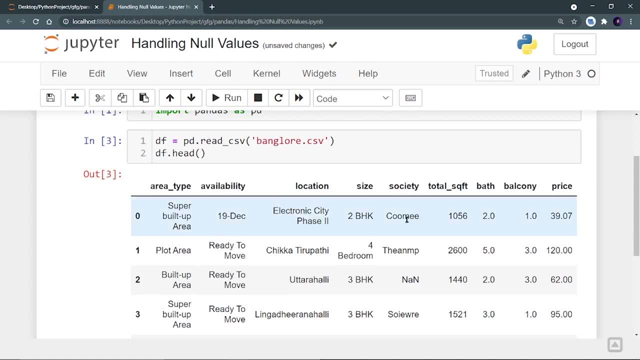 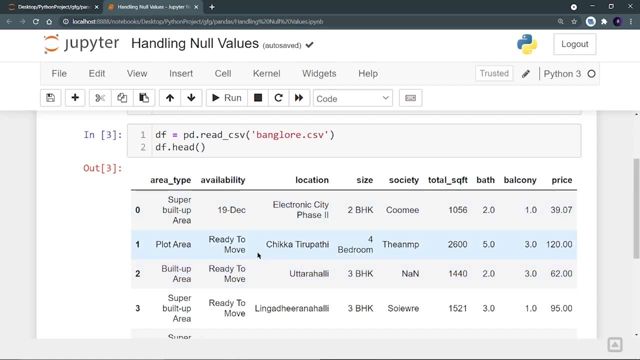 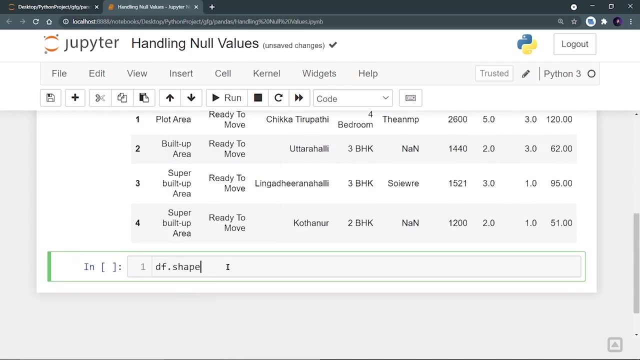 Let's run it And I can see the columns, the features of this dataset, And let's say we have to analyze this complete dataset. So for that, first of all, we need to check what is the shape of this dataset. We can do dfshape, So this is going to return me a tuple which will tell the rows, columns. 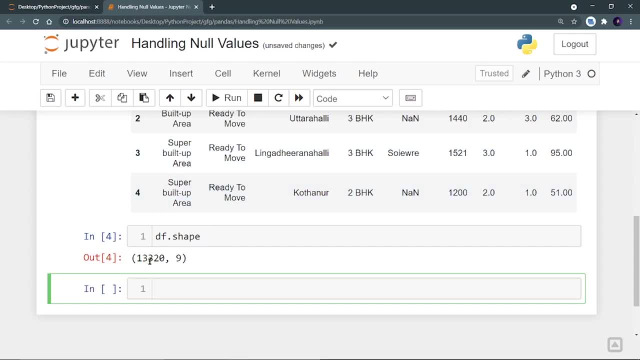 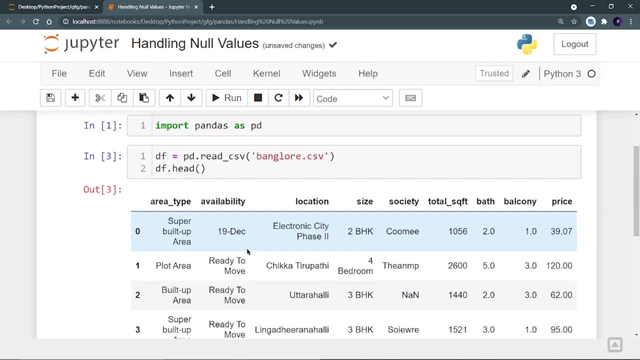 So this means that this complete CSV file contains 13,320 rows and nine columns, And you can also see that 1,, 2,, 3,, 4,, 5,, 6,, 7,, 8, and 9 columns are there right Now. this. 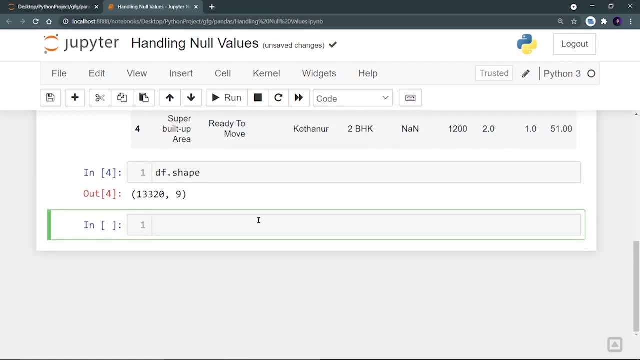 dataset may contain some null value, right? So we have to analyze it. So for that there is a function called dfisNull, Right. This function is going to return me true or false. So it returns basically the boolean value. So wherever in this dataset the null value will be there, then it will be true. 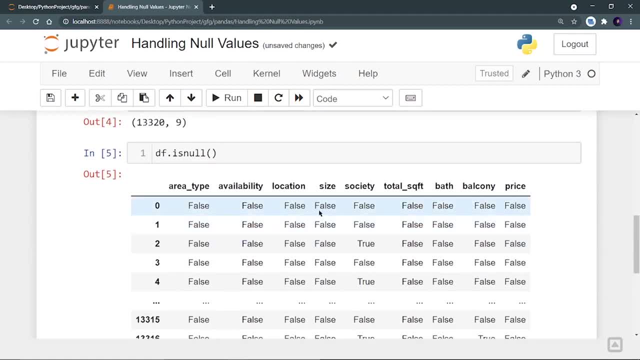 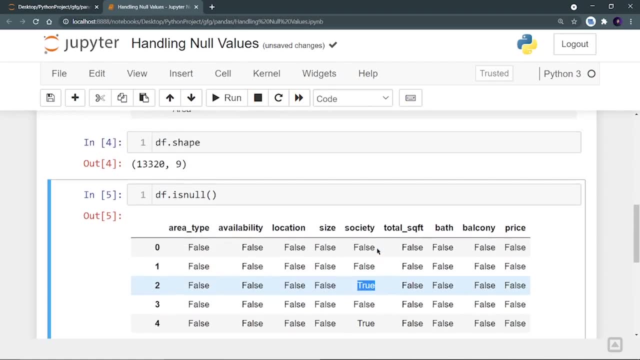 either it will be false, right, So let's run it. So I can see that mostly it is false, but I can see some places. at some places it is true. So this true means the value at this cell is null, right, You can also see over. 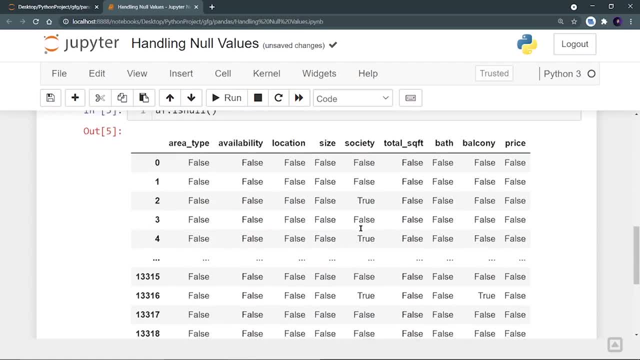 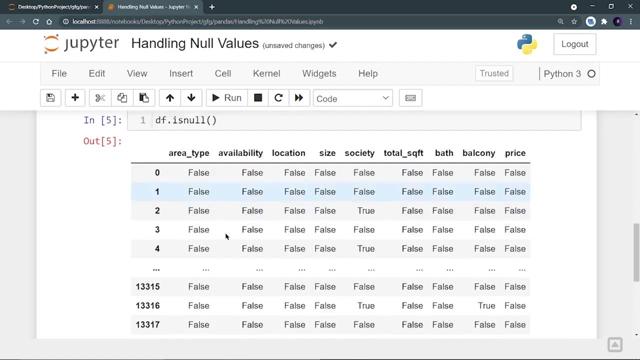 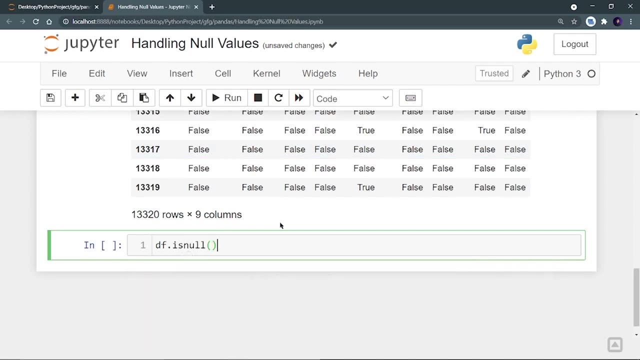 here it is Nn. Nn means null. right Now, I don't want this complete, true, false, true, false thing. I want a total number, right For every column. So for that thing, what you have to do is you have to run a function called dfisNullsum, and let's run it So, column wise. 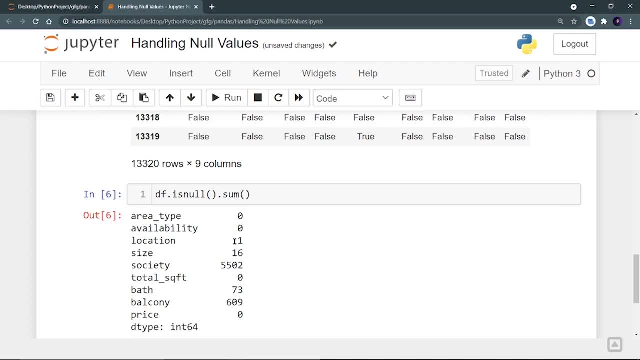 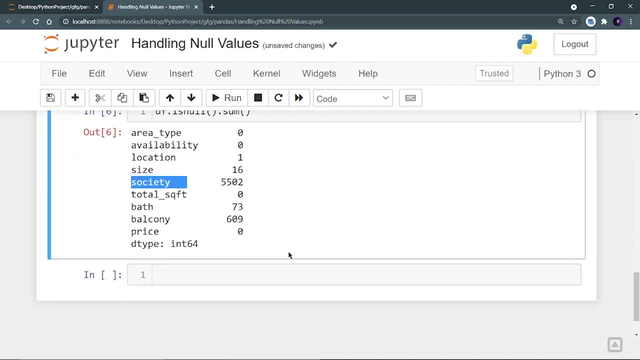 it is giving me that area type column contains zero null values, location contains one null value, size contains 16 null values and society column contains 5,502 null values. right, So this gives me the total sum of the null values in each column. 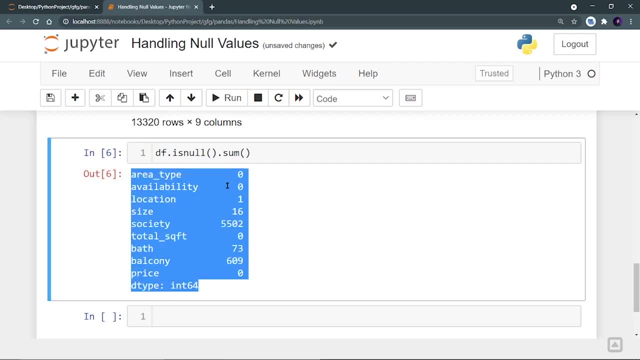 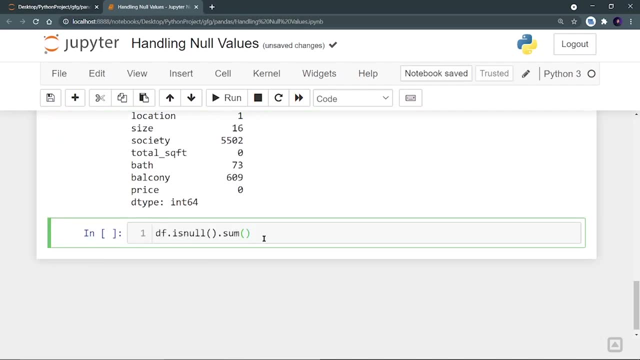 Now, you don't want it to be in column wise. also, I want a final number, I want a scalar value, just a number, right. So for that thing, you will just copy this line and you will paste it and you will do a sum of this also, right? So let's do a sum and let's see So: total: 6,201. 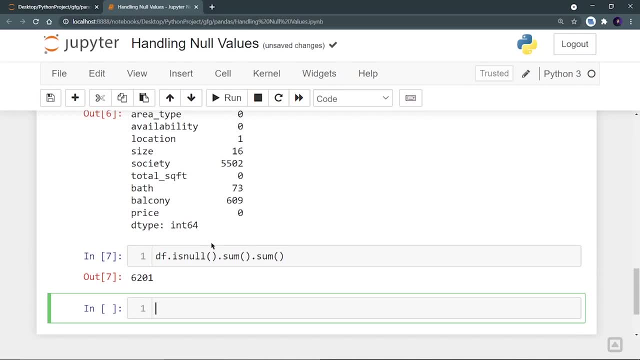 null values are there in my dataset- Perfect. Now, what is my task? My task is to fill this thing with the null values. Now, what is my task? My task is to fill this thing with the null values. Now, what is my task? My task is to fill this thing with the null values, Or we can drop these null. 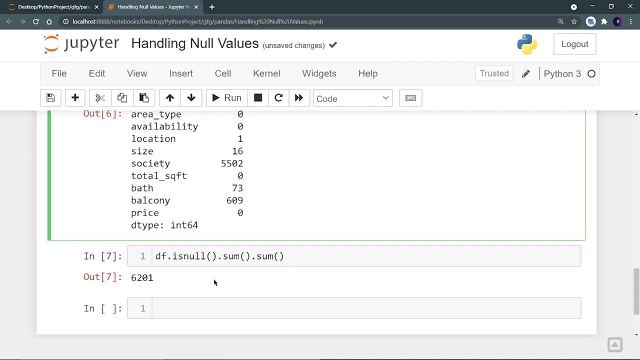 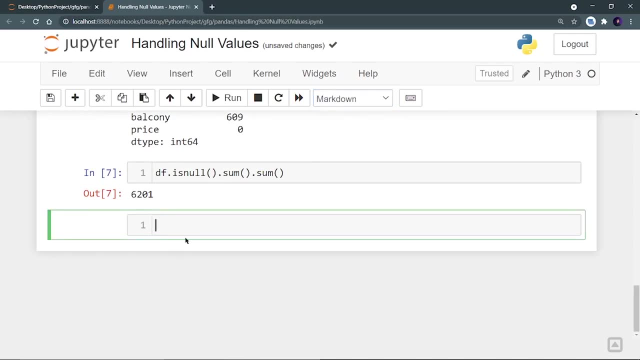 values. we can remove these null values or we can either replace these null values with some other number, right? So first thing that we are going to see, let's put a markdown and over here I'm going to put: filling the null values. filling null values, Let's put it this way: Yes. So first, 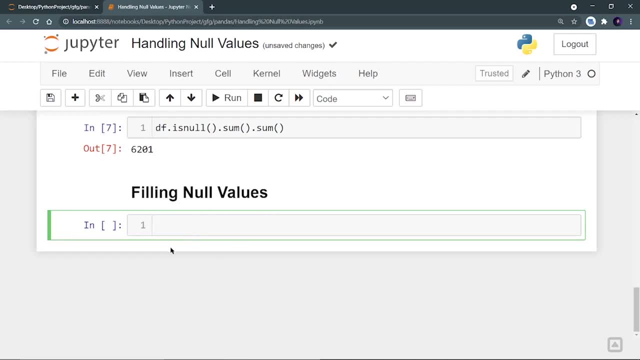 thing we are going to do, how we can fill this null values. So for filling the null values, we can use an inbuilt function called fillna, and that we can use it by writing dffillna, and you have to provide a value in this as a parameter. So this value equal to zero means wherever the null values. 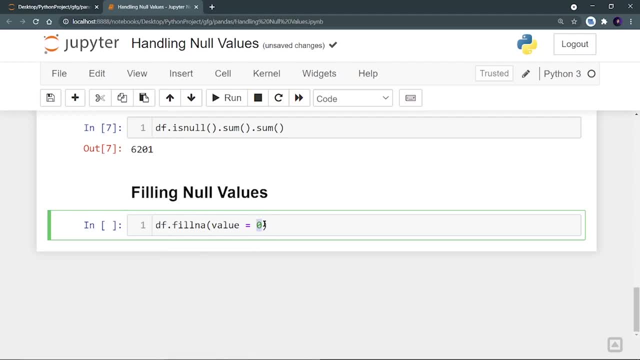 will be present in my dataset. zero is going to replace them, right. And now we are going to create a new data frame called df2 and it is going to contain my new data frame, right, Because I don't want to affect the original data frame that is containing the null values, right? So 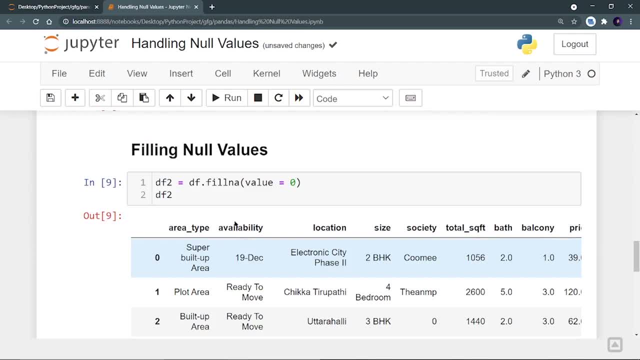 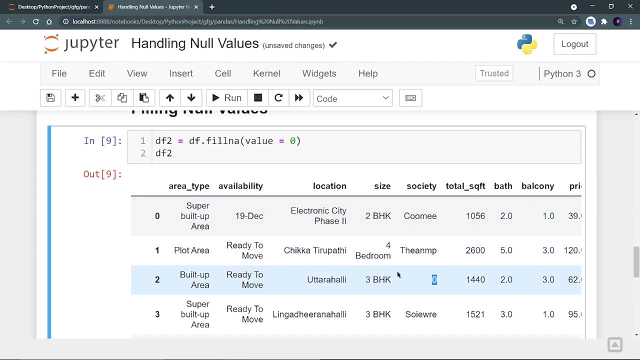 now let's check df2 and let's run it. So I can see that at this point it was a null value in the df. but here in df2, I can see that it is zero and everywhere, wherever it will be true. that means 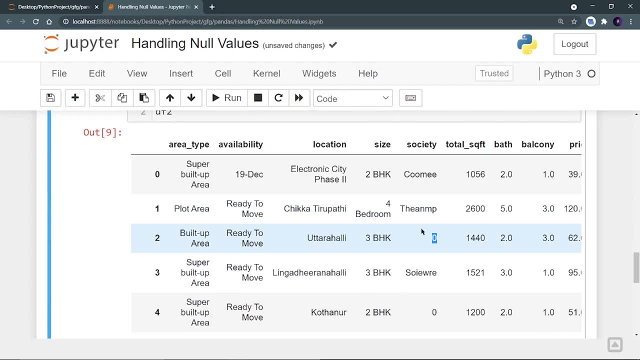 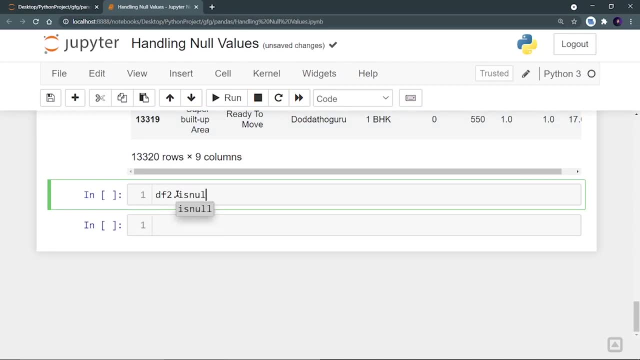 wherever it was a null value. now in this df2, it contains zero. Let's check it whether df2 contains any null value or not. So what I'm going to do, df2.isNullsum sum and when I'm going to run it I can see that zero. but if I run dfisNullsumsum, 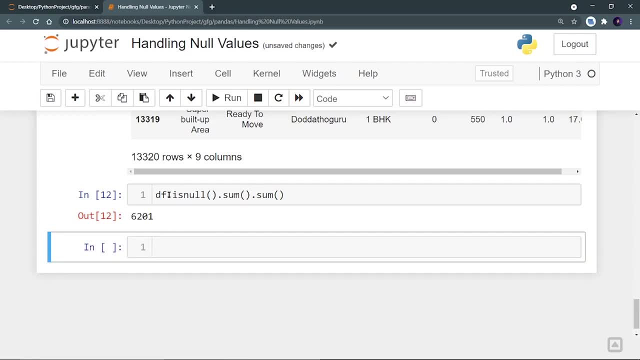 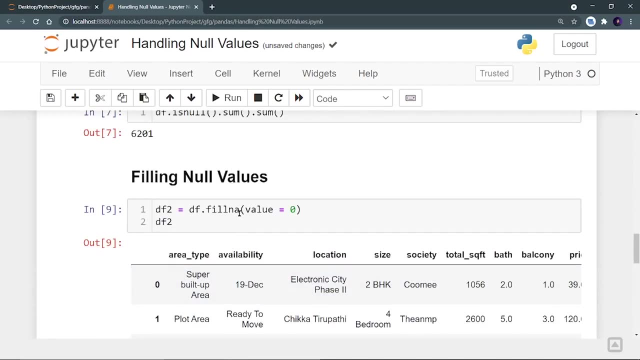 I can see that again. 6,201 values are there in the original df, but in df2, there is no null value. Why? Because I have filled those null values with zero. So this is how you can fill in all values. 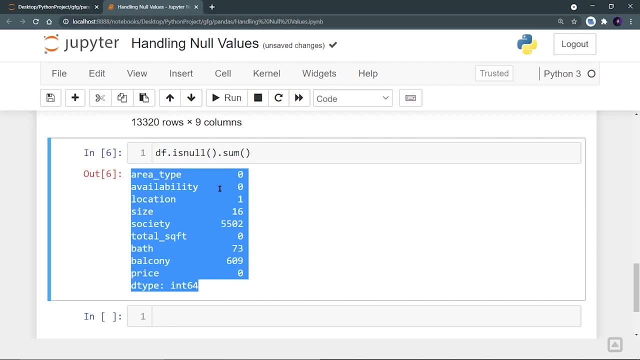 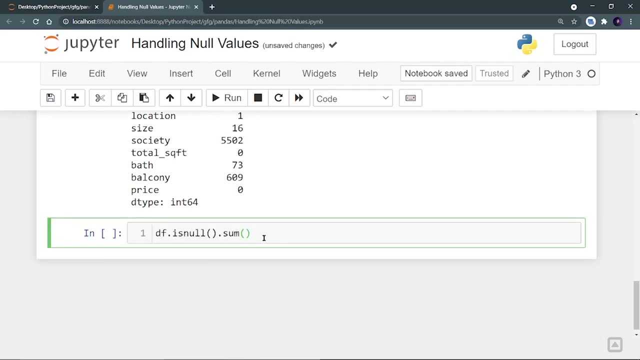 you don't want it to be in column wise. also, I want a final number, I want a scalar value, just a number, right. So for that thing, you will just copy this line and you will paste it and you will do a sum of this also, right? So let's do a sum and let's see So total. 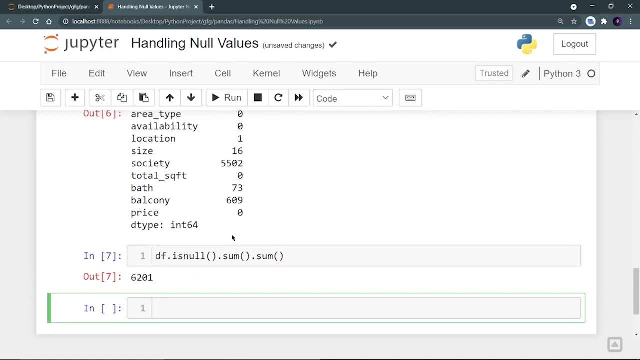 6,201 null values are there in my dataset- Perfect. Now what is my task? My task is to run a function called dfisNullSum and let's run it. So I'm going to run a function called dfisNullSum. My task is to fill this null values, or we can drop these null. 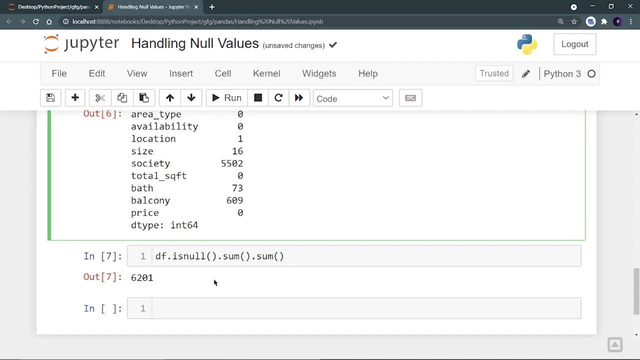 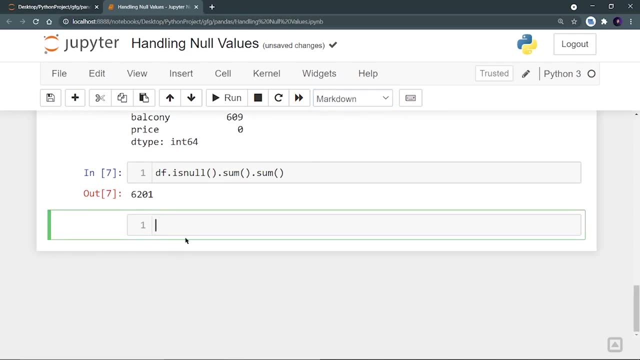 values. we can remove these null values or we can either replace these null values with some other number, right? So, first thing that we are going to see, let's put a mark down and over here I'm going to put: filling the null values. filling null values, Let's put. 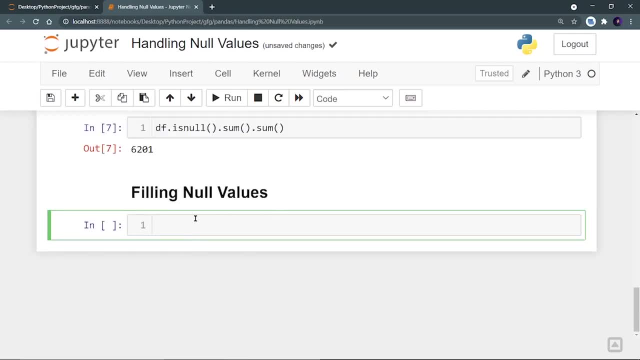 it this way? Yes, So first thing we are going to do how we can fill this null values. So for filling the null values, we can use an inbuilt function called fillna, and that we can use it by writing dffillna, and you have to provide a value in this as a parameter. 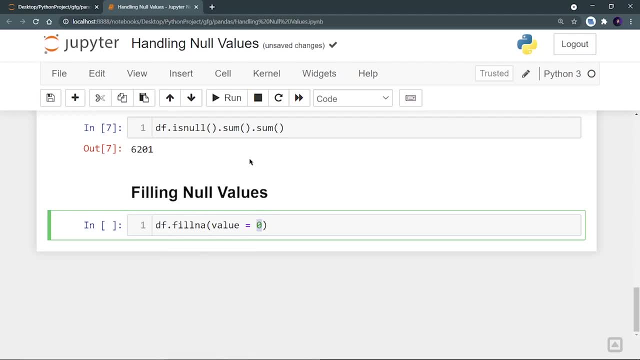 So this value equal to zero means wherever the null values will be present in my dataset, zero is going to replace them, right? And now we are going to create a new data frame called df2 and it is going to contain my new data frame, right, Because I don't want to. 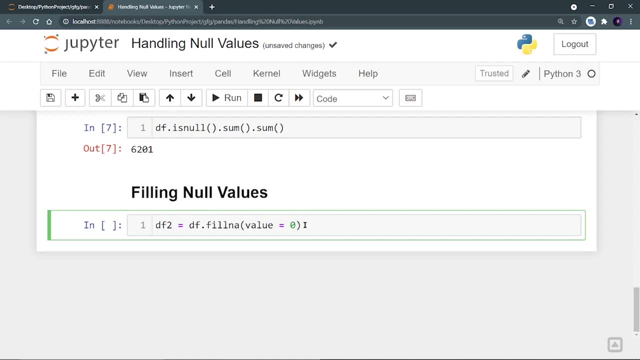 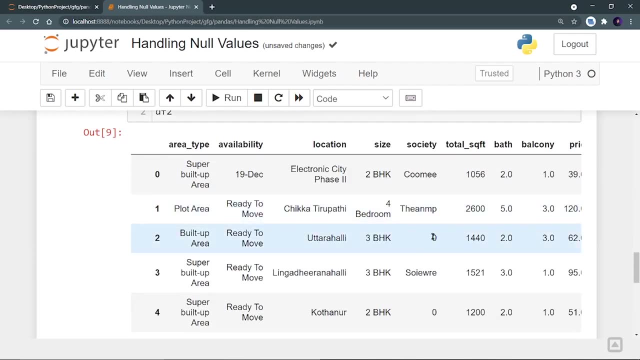 affect the original data frame That is containing the null values, right. So now let's check df2 and let's run it. So I can see that at this point it was a null value in the df, but here in df2, I can see. 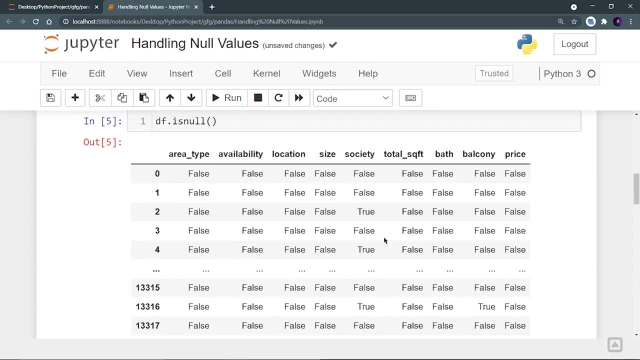 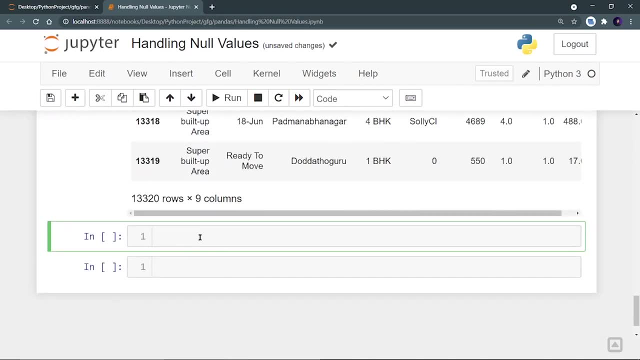 that it is zero, and everywhere, wherever, it will be true. that means wherever it was a null value. now in this df2, it contains zero. Let's check it whether df2 contains any null value or not. So what I'm going to do: df2.isNull, right. 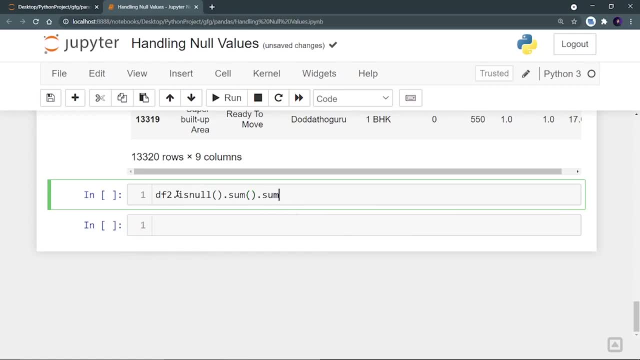 df2.isNullsumsum, and when I'm going to run it I can see that zero. But if I run dfisNullsumsum I can see that again. 6,201 values are there in the original df, but in df2, there is no. 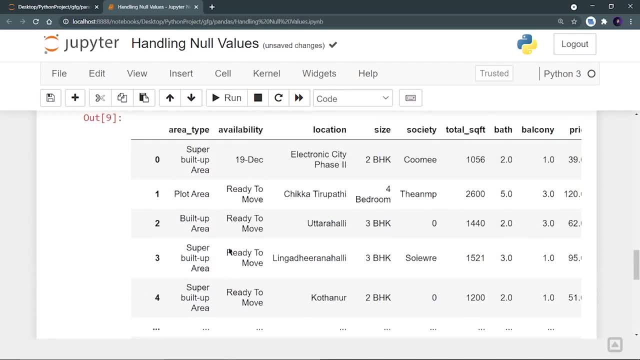 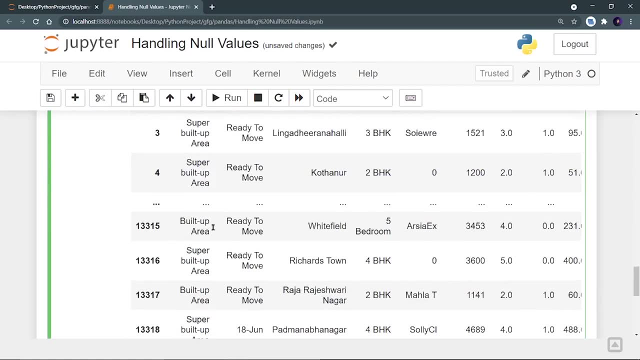 null value. Why? Because I have filled those null values with zero. So this is how you can fill the null values. Let's do one more thing. Let's fill it with some another value. Let's fill it with: let me copy it, Let me paste it And let's make it a null. Let's 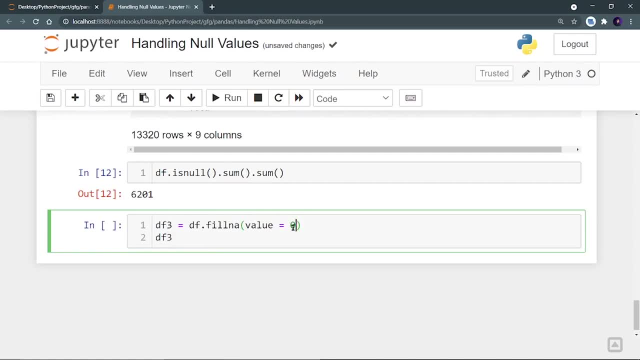 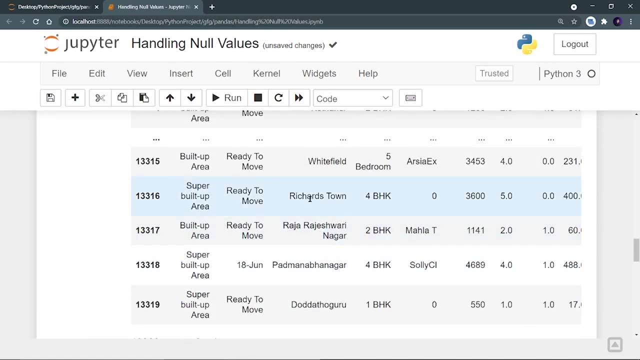 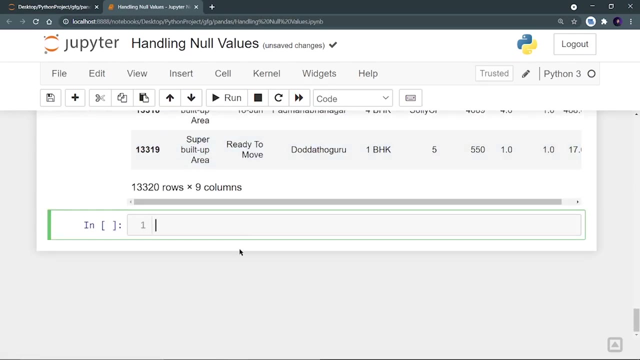 make it df3 and let's fill it with 5.. So I can see that instead of zero, it has now filled it with 5.. Perfect, So now you know that what is dfisNull? sorry, dffillna. right Now let's do one more experiment with dffillna. So this is my original data frame: df, and. 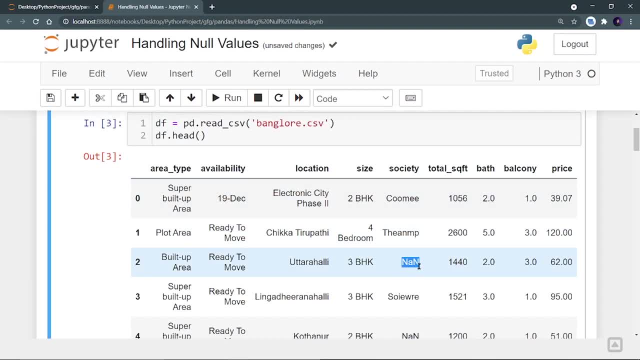 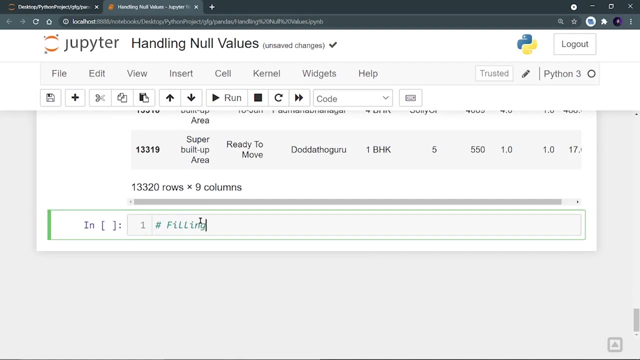 here is one of my null values. Now what I want to do. I want to fill this null value with just a previous value, like this: I want to fill this null value with the previous value. Now how I can do it. So let's put a topic, Let's put a comment: filling null values. 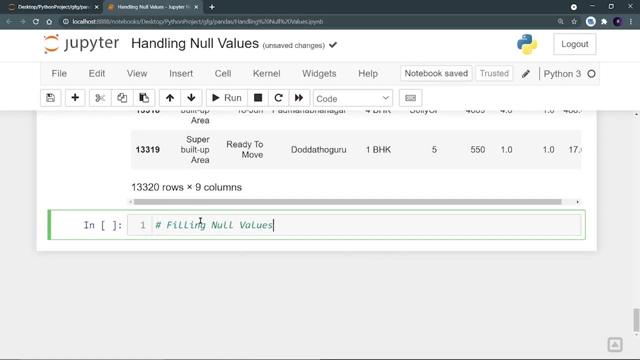 with previous value. right Now. you have to define just another parameter. So let's create a new data frame for df4.. df4 is equal to dffillna and you have to define a method, And my method will be. you have to define pad. that is pad, right? So it is going to fill the null values with just. 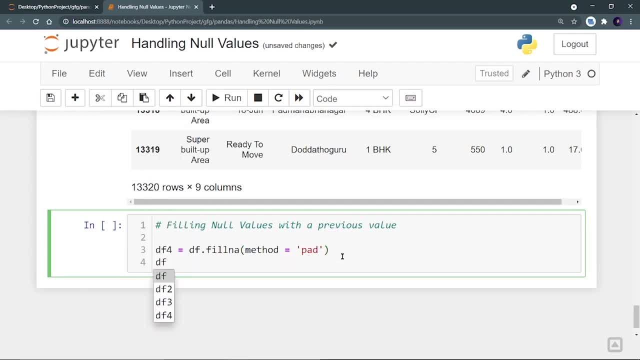 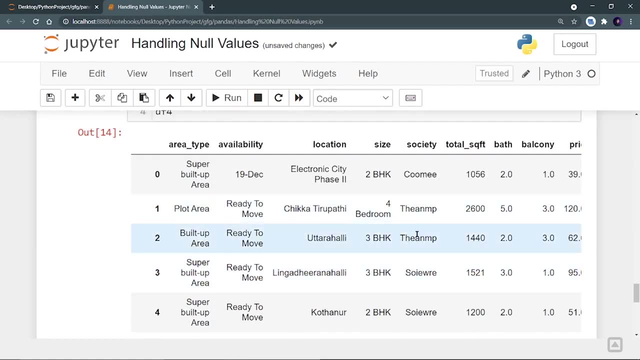 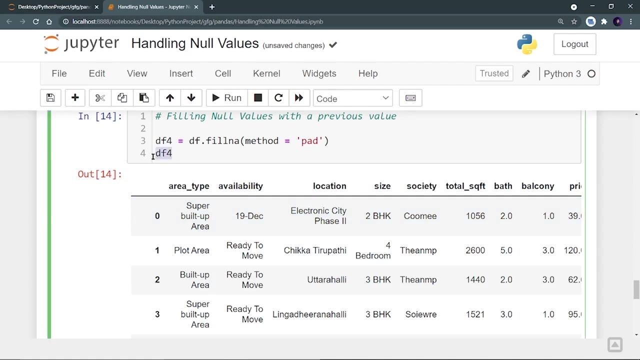 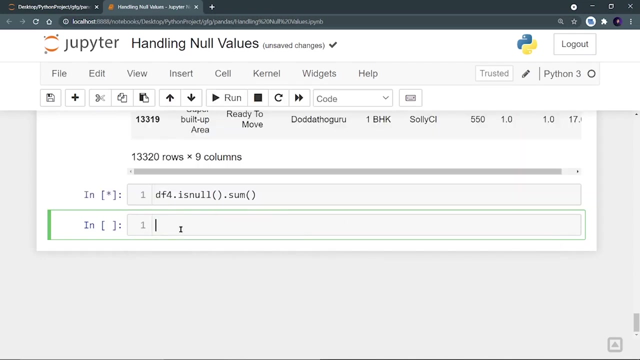 a previous value. Now let's run it. So let's print df4 and let me run it, And I can see that where it was null, it is now filled with the previous value. Now what I want to do? now let's do a quick verification whether my df4 contains any null value or not. So df4.isNullSum. 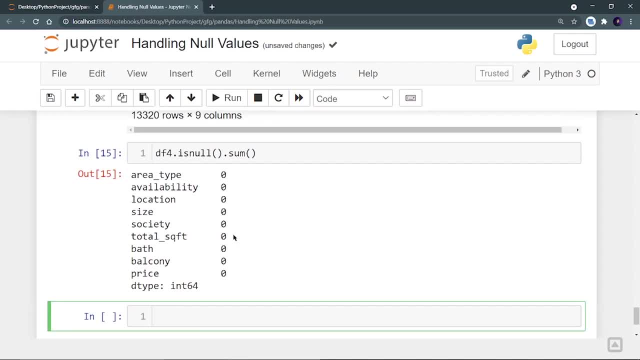 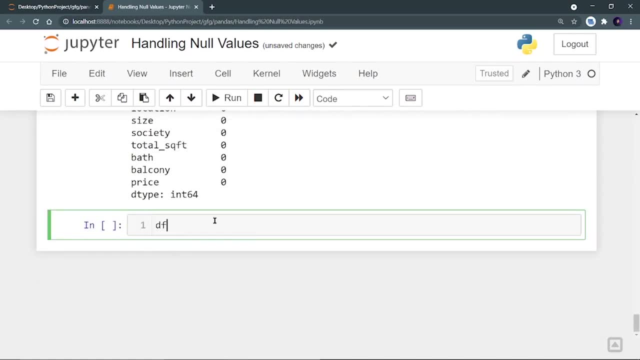 I can see that none, no, no column of this df4 contains any null value. Perfect. Now the next task is to fill the null values. Let's first of all print df, which is my original data frame. I can see that it is having the null values. Now we have seen how we can fill. 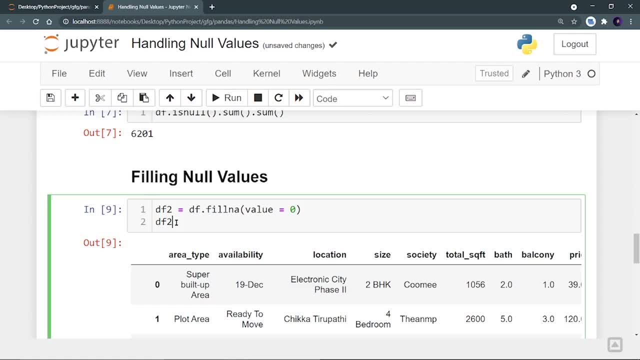 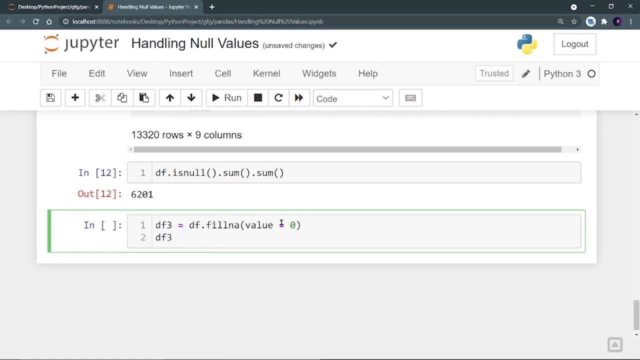 Let's do one more thing. Let's fill it with some another value. Let's fill it with: let me copy it. Let me paste it and let's make it df3.. And let's fill it with 5.. So I can see that instead of zero, it has now filled it with. 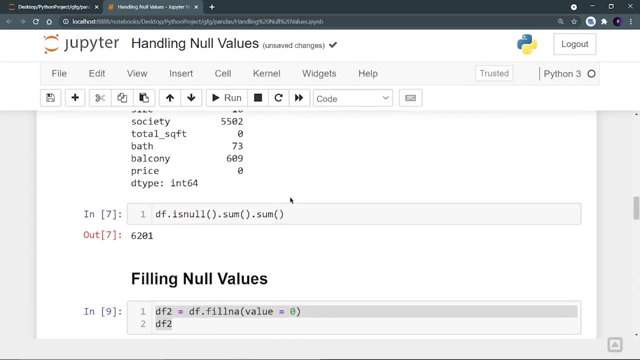 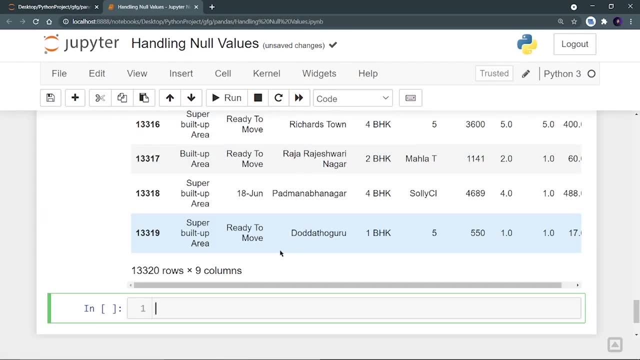 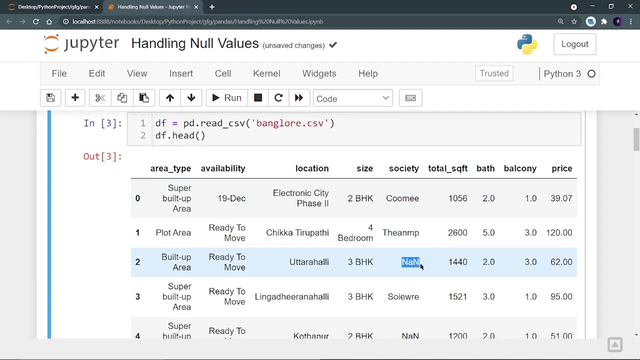 5. Perfect. So now you know that. what is dfisNull? sorry, dffillna. right Now let's do one more experiment with dffillna. So this is my original data frame df, and here is one of my null values. 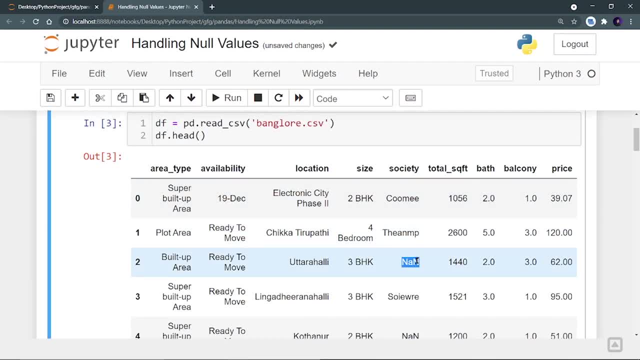 Now what I want to do. I want to fill this null value with a just a point. I want to fill this null value with a just a point. Now what I want to do. I want to fill this null value with a just a point. 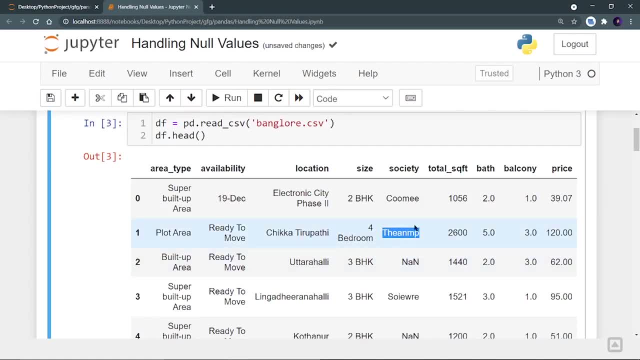 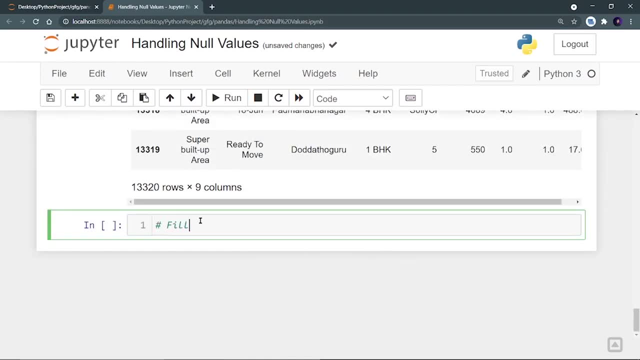 Now what I want to do. I want to fill this null value with a just a point Like this. I want to fill this null value with the previous value. Now how I can do it? So let's put a topic, let's put a comment filling null values. 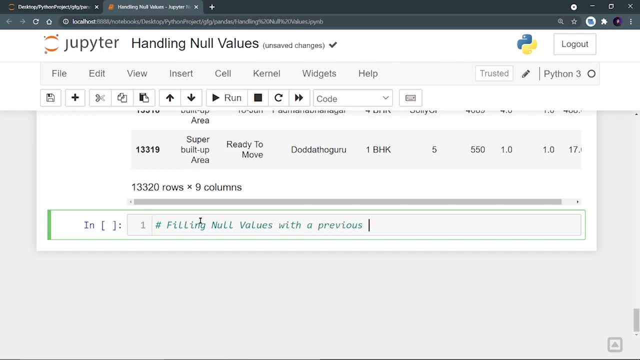 with previous value. Right Now, you have to define just another parameter. So let's create a new data frame, for df4 is equal to dfisNull fillna, and you have to define a method, And my method will be: you have to define pad. 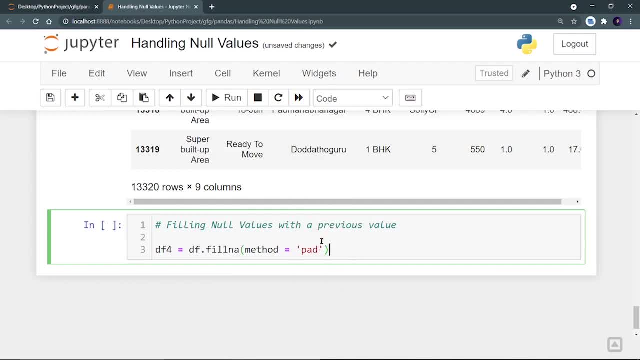 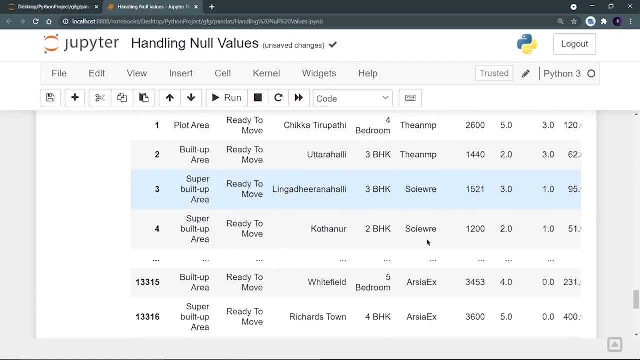 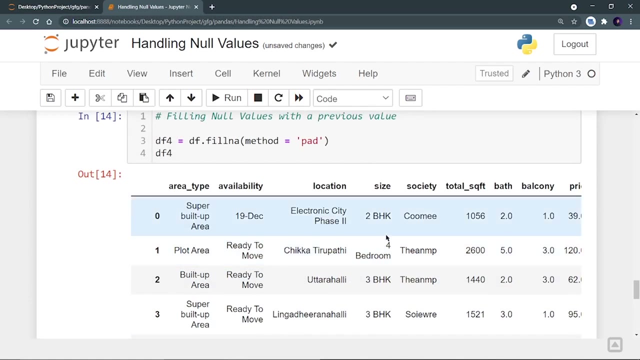 that is pad right. So it is going to fill the null values with just a previous value. Now let's run it. So let's print df4 and let me run it, And I can see that where it was null, it is now filled with the previous value. Now what I want to do? now let's do a quick verification for. 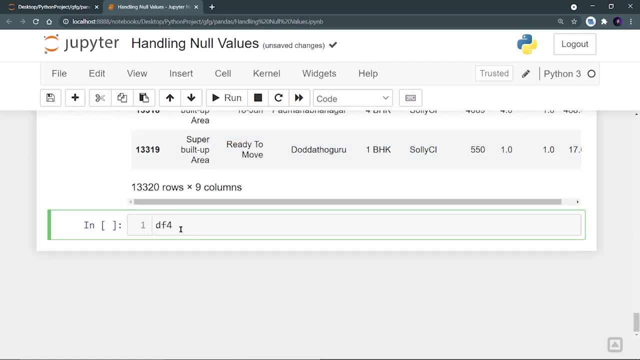 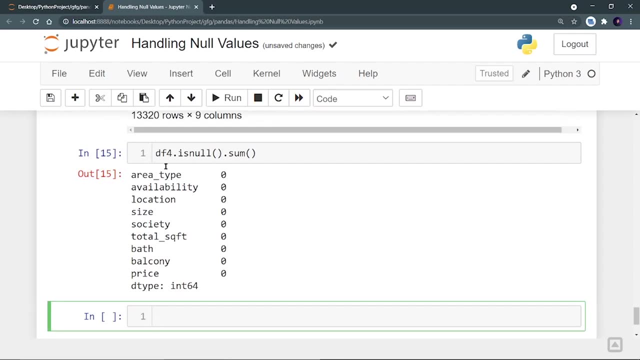 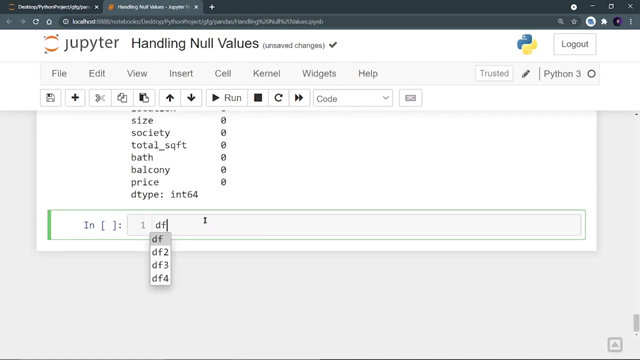 whether my df4 contains any null value or not. So df4.isNullsum. I can see that none, no, no column of this df4 contains any null value. Perfect, Now the next task is to fill the null values. Let's first of all print df, which is my original. 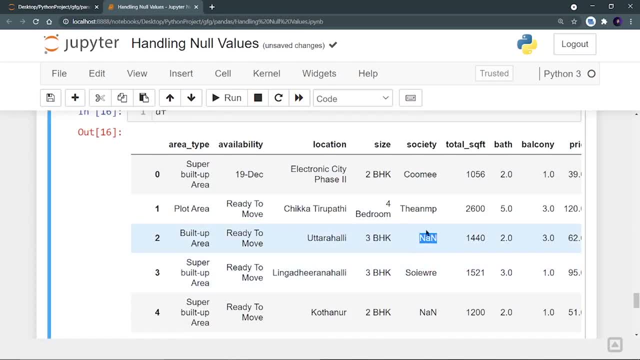 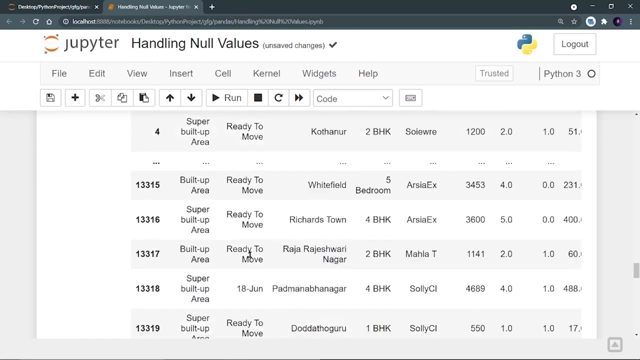 data frame, I can see that it is having the null values. Now we have seen how we can fill this null values with the previous value. Now I want to fill this null value with the coming value or the next value, row-wise. right So, next row value. I want to print over here, right So what I can, what I 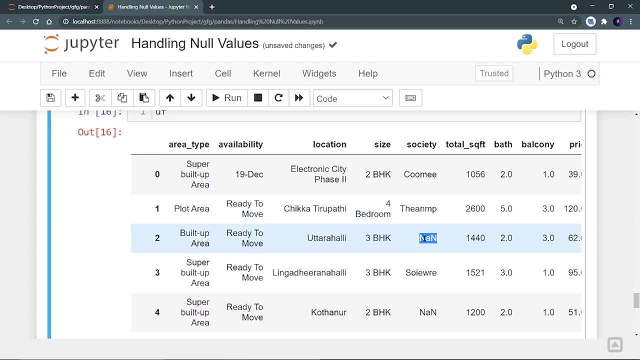 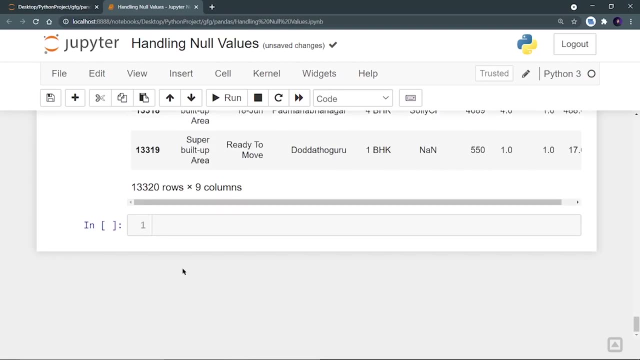 this null values with the previous value. Now I want to fill this null value with the coming value or the next value row wise, right So? next row value. I want to print over here, right? So what I can, what I can do, is let's copy the same thing, Let's paste it over here. 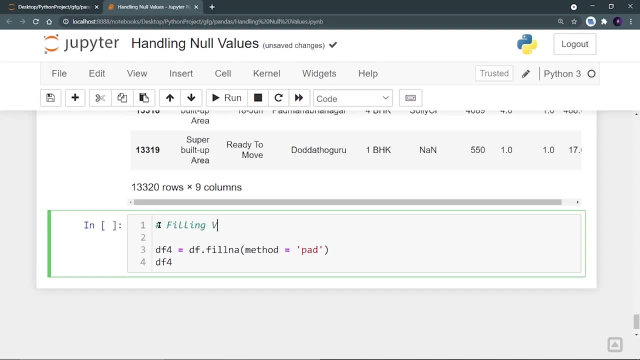 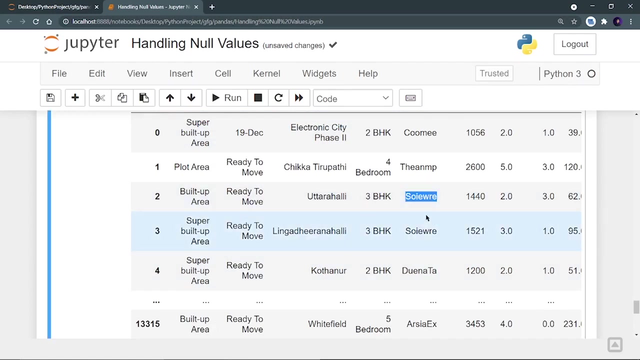 Now my topic is filling null values with the next value. Okay, Okay, Right, So let's create df5.. Method is going to be BFILL, That is, backward fill. Right, So let's run it. And I can see that instead of the null value, I'm getting the next value. 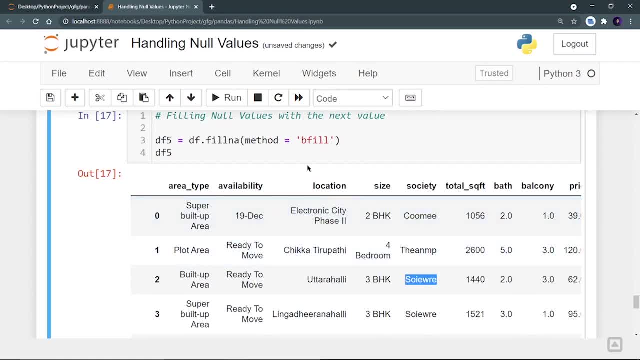 row wise. Perfect. So we have seen how we can fill these null values using pad method, using backward fill method, Right? So let's do a quick recap of these two methods. In pad method, we fill the null values with the previous value, row wise, but in the BFILL, that is. 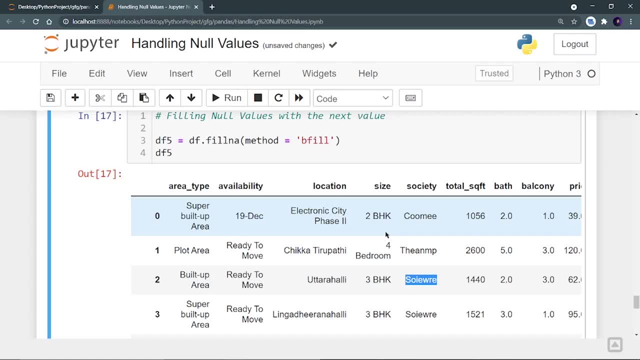 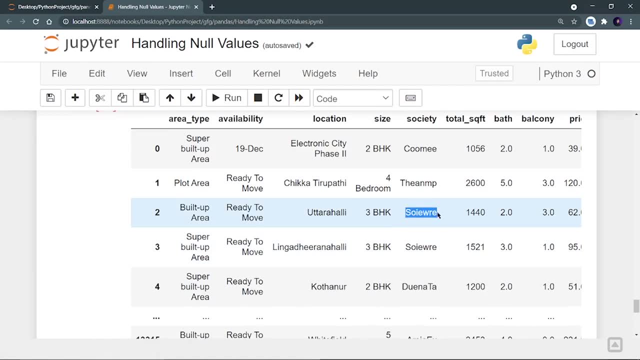 backward fill. we fill the values with the coming value, right With the next value, row wise. Right Now we have seen filling the null values called row wise. right, What I was doing? I was filling this null value. Let me come to df. I was filling this null value with 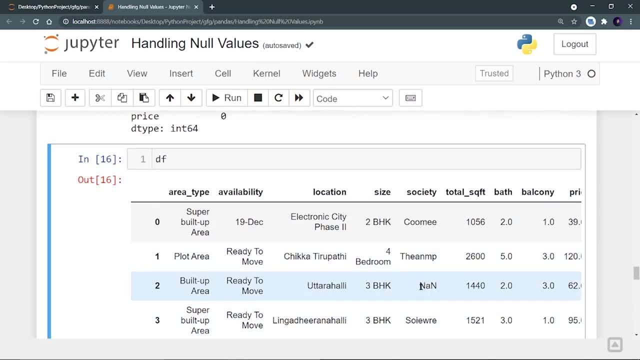 this value by pad and this value by backward fill. But now I want to fill this null value with a previous value, but column wise. Or the second method will be filling this null value with a coming value- column wise, right? So let's see how we can do it. We don't have 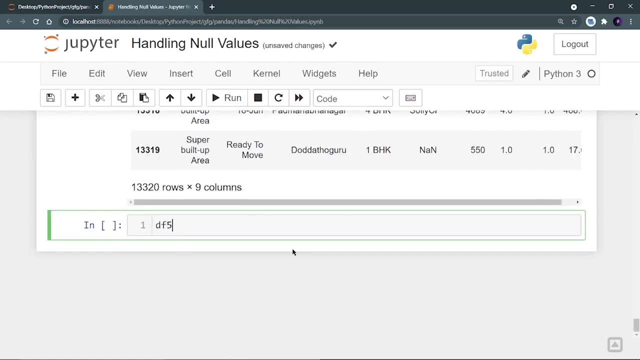 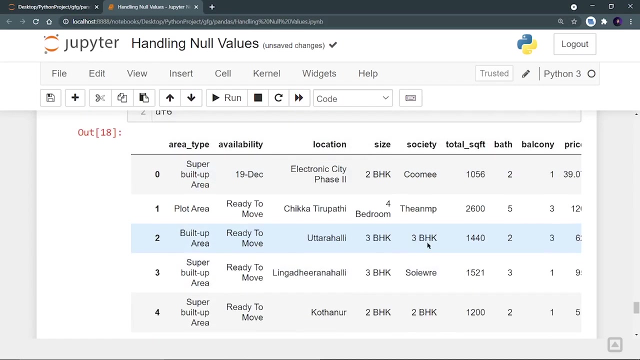 to do something unique. We just have to define fillna-only. df. 6 is equal to dffillna. method is going to remain the same, That is pad, But my axis will be 1.. Let's print df6 and I can see that my null value is filled with the previous value. but 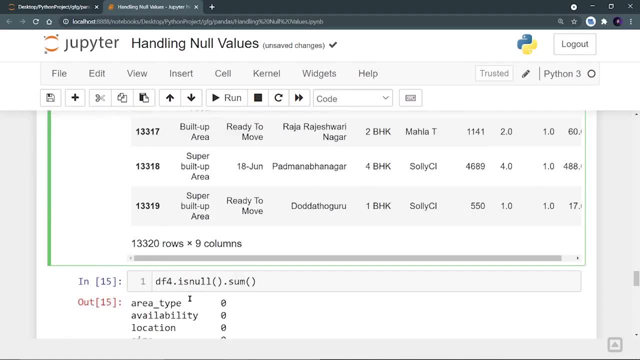 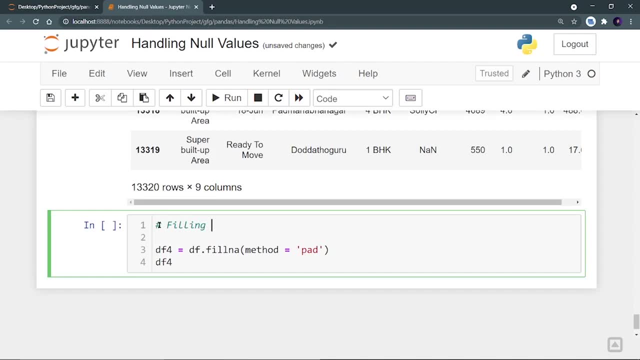 can do is: let's copy the same thing. Let's paste it over here. Now, my topic is filling null values with the next value, right? So let's run the next activity. right, So let's create df5,. method is going to be bfill, that is, backward fill, right? 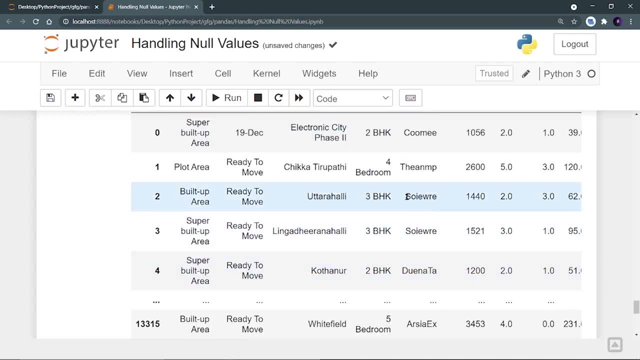 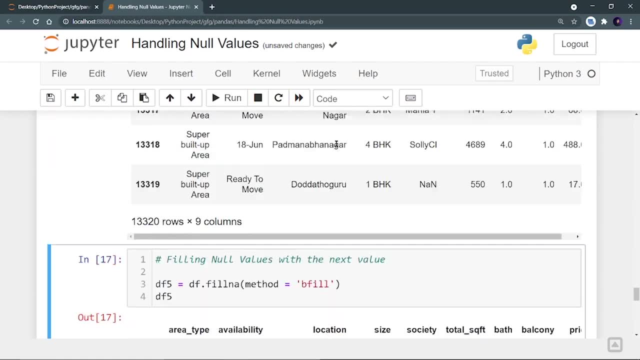 So let's run it And I can see that, instead of the null value, I'm getting the next value row. wise, perfect. So we have seen how we can fill these null values using pad method, using backward fill method, right? So let's do a quick recap of these two methods. 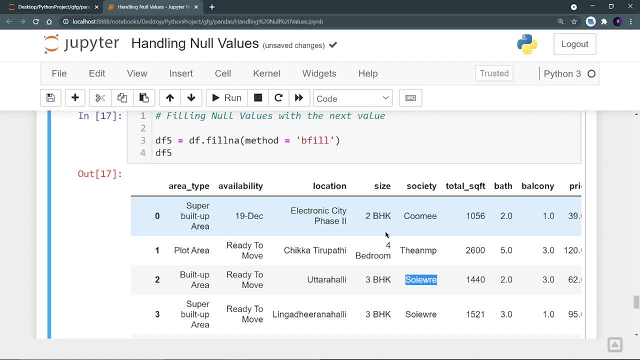 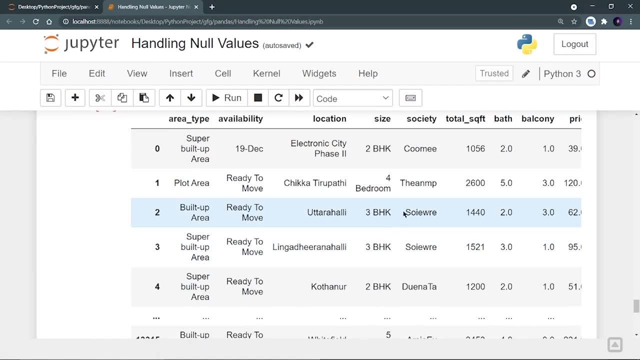 First row wise. but in the bfill, that is backward fill, we fill the values with the coming value right With the next value, row wise right. Now we have seen filling the null values, called row wise right. What I was doing, I was filling this null value. 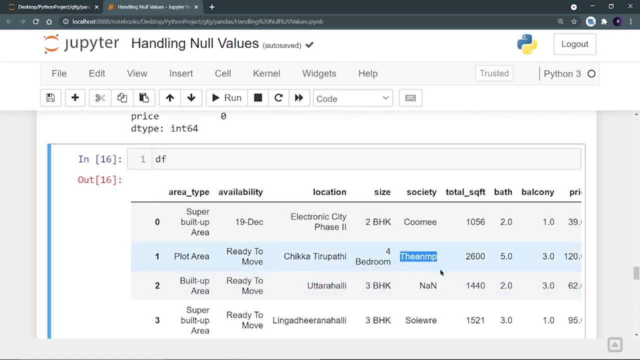 Let me come to df. I was filling this null value with this value by pad and this value by backward fill. But now I want to fill this null value with a previous value, but column wise. or. the second method will be filling this null value with the coming value, column wise, right. 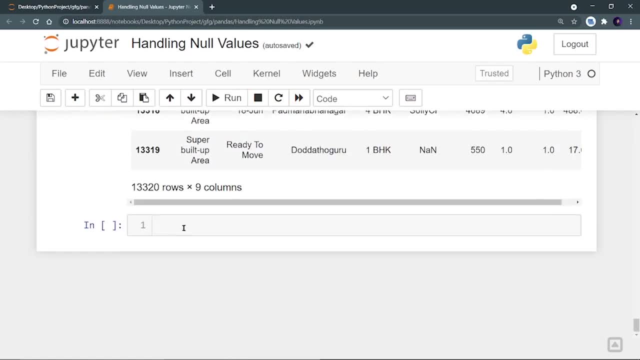 So let's see how we can do it. We don't have to do something unique, We just have to define fillna. only. df6 is equal to dffillna. method is going to remain same, that is pad, But my axis will be 1.. 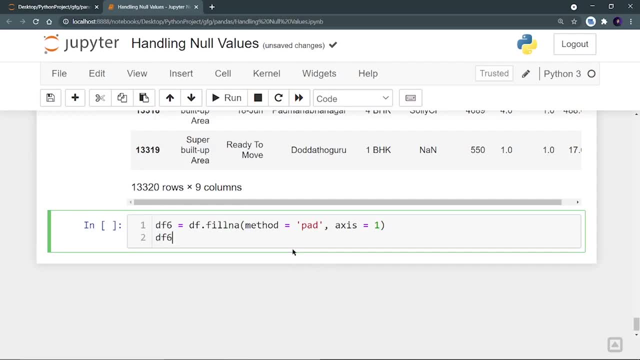 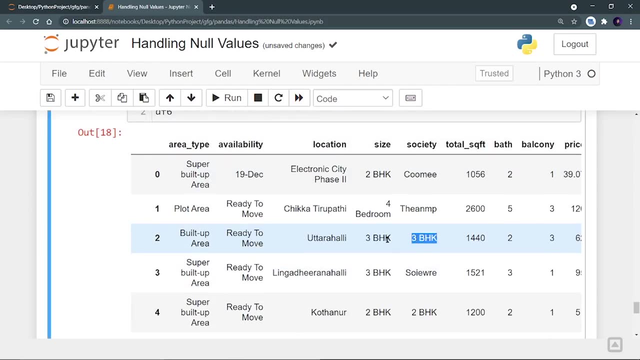 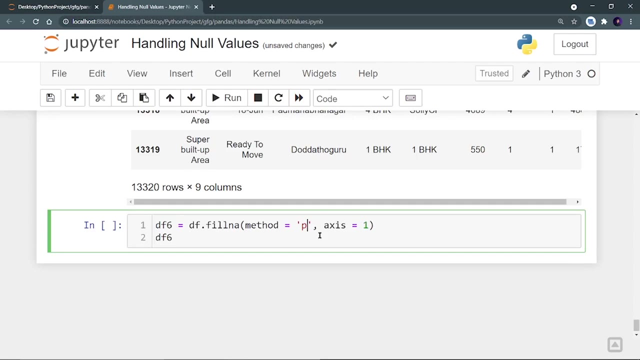 Let's print df6.. And I can see that my null value is filled with the previous value. but, column wise, Let's do the same thing And let's make the method as bfill, and let's change the data frame number and let's print: 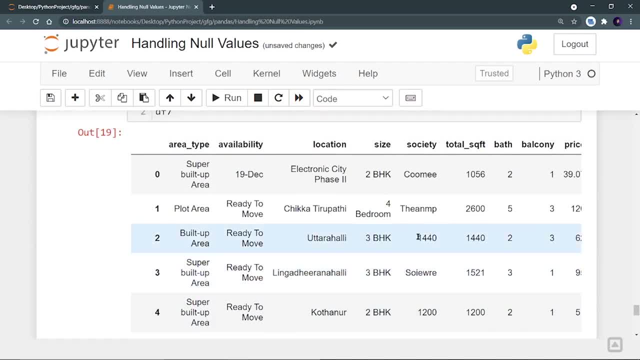 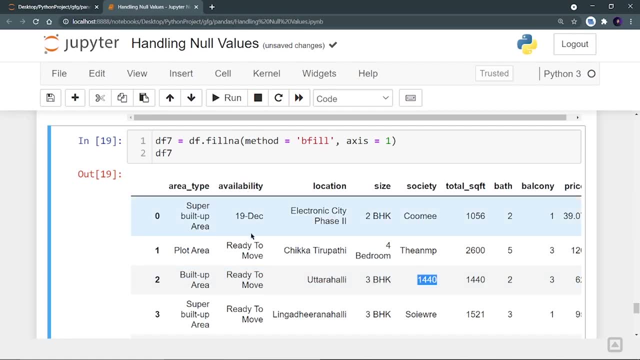 it. And here I can see that the null value is filled with the coming value. but column wise. So this was how you can fill the column. Let's fill the values: a previous value or the next value. Now we have something more in fillna method. 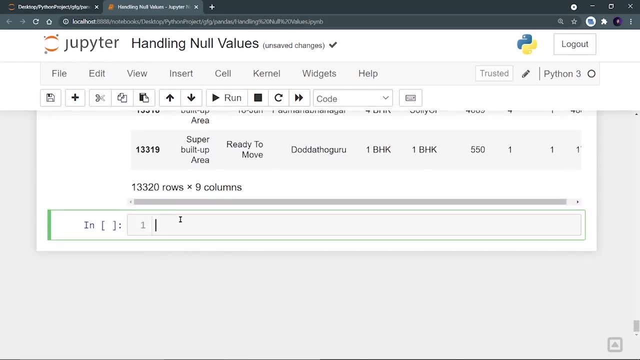 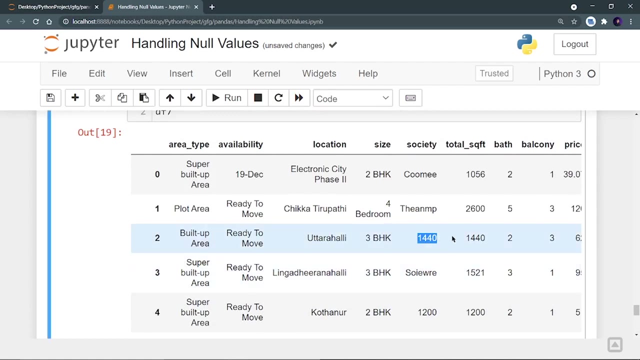 column wise, Let's do the same thing and let's make the method as bfill and let's change the data frame number and let's print it, And here I can see that the null value is filled with the coming value. but, column wise, 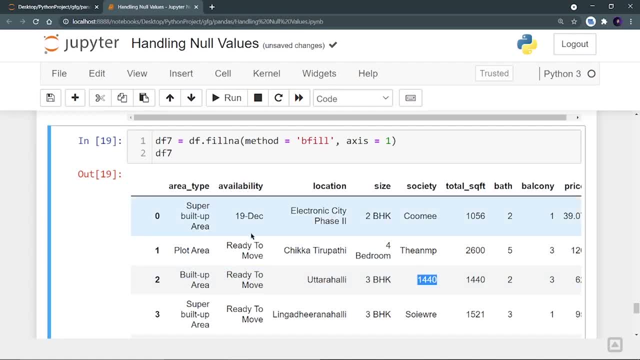 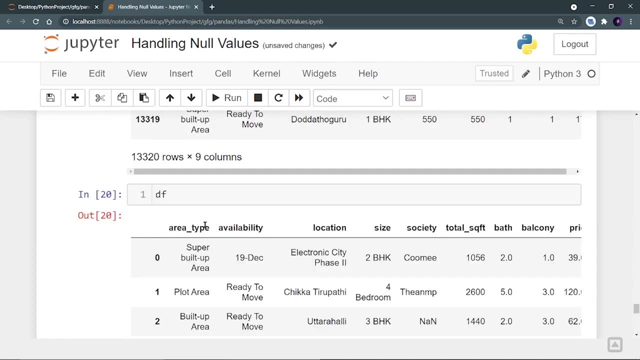 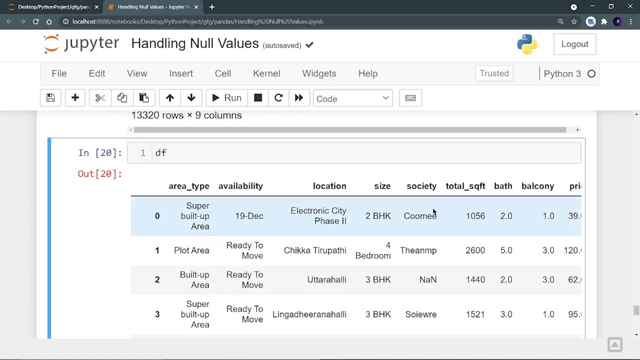 So this was how you can fill the values: a previous value or the next value. Now we have something more in fillna method. Let's see the df first. So this is my original data frame. Now what I want to do is, my task is to fill a null value only, but I want to fill a different. 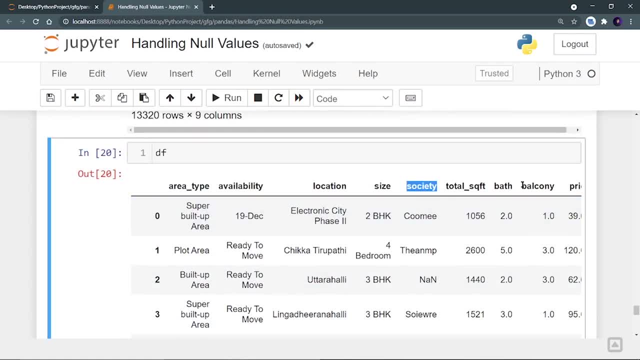 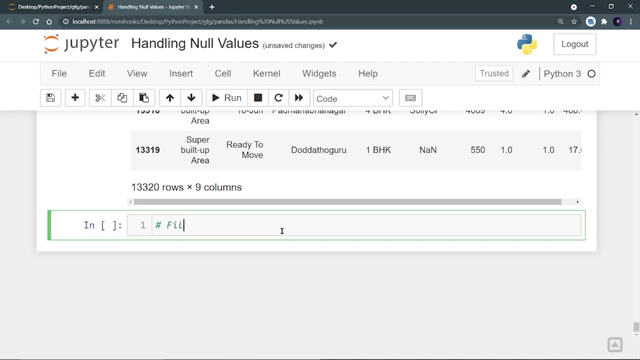 value in society column and a different value in this balcony column. right Now, how I can achieve it: You have to do fillna only. So let me put the command filling null values, filling different null values, filling different values in null in different columns. 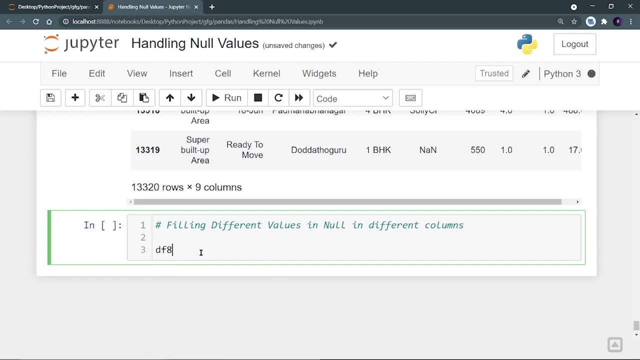 So what I can do is you have to write df. let's create: df8 is equal to df, Fillna and over here. you have to define a dictionary and inside this dictionary, you have to define a key which will be your column name. 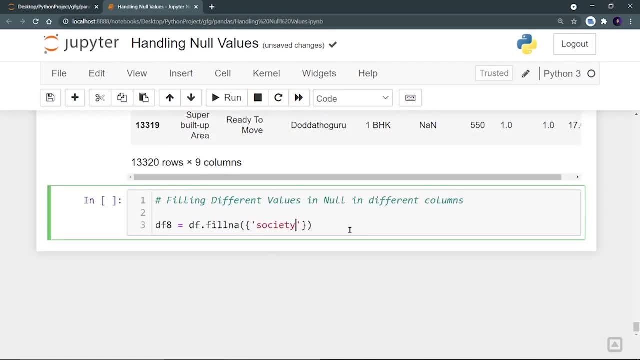 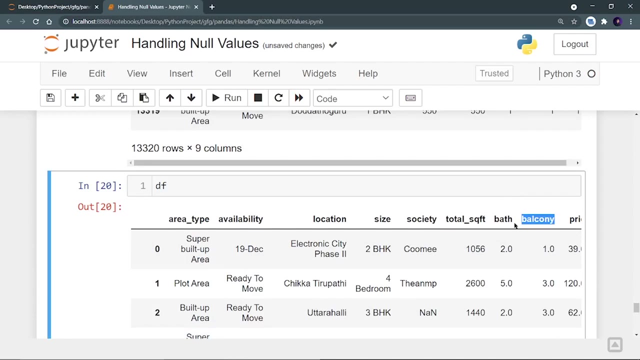 So let's take the column name as society and in society. you want to fill this with, let's say, abcd, right? So let me put it in a string: abcd. and the second column name is balcony, So let's copy it and paste it. 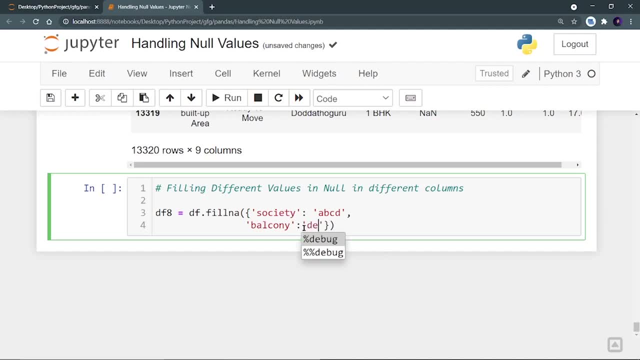 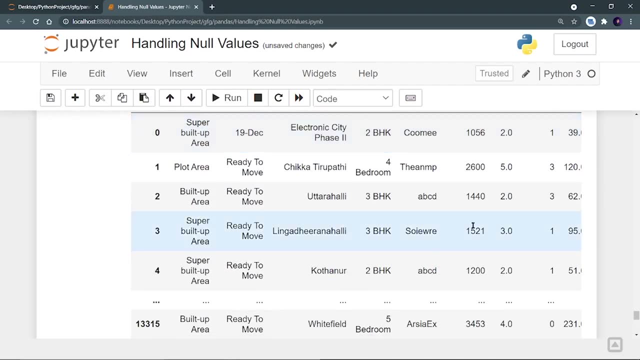 And here you want to fill the null value with defg. right, Let's print df8 and let's see what we have got So over here I can see that in society my null value is filled with abcd and in balcony. 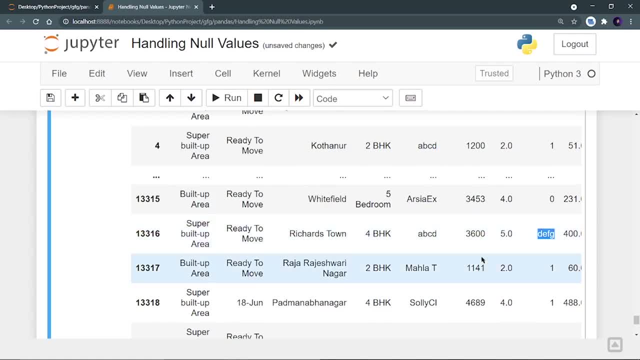 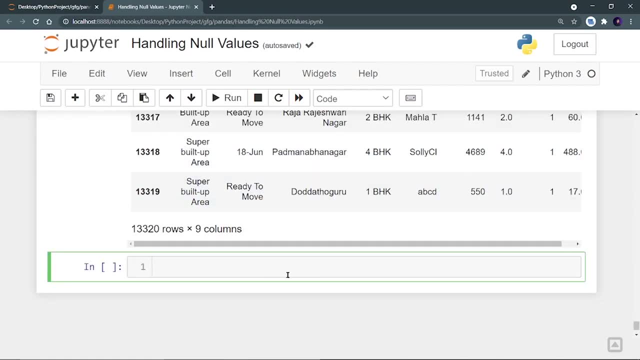 my null value is filled with defg. So here I can see that how I am filling the null values for different, different columns. right Now, let's see the next thing Now here. what I want to do is I want to fill the null value with the mean of the complete column, right? 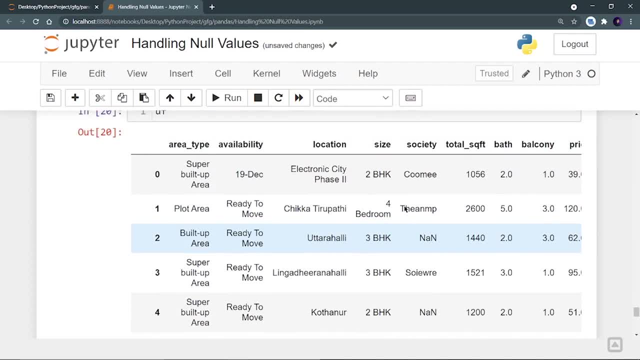 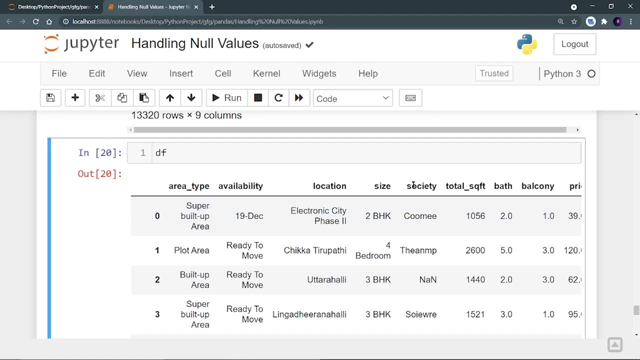 Let's see the df first. So this is my original data frame. Now what I want to do is my task is to fill a null value only, but I want to fill a different value in society column and a different value in this balcony column, right. 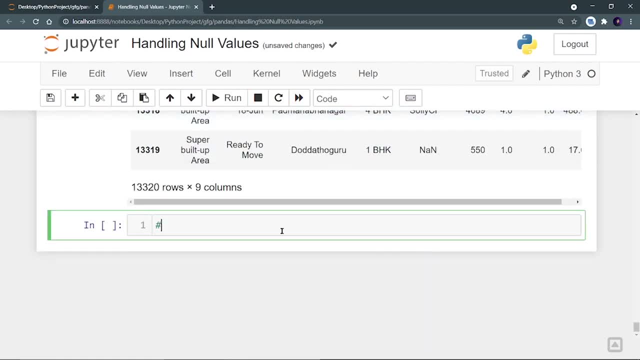 Now how I can achieve it. You have to do fillna only. So let me put the comment filling Null values, filling different null values, filling different values in null in different columns. So what I can do is you have to write df. let's create df8 is equal to dffillna. 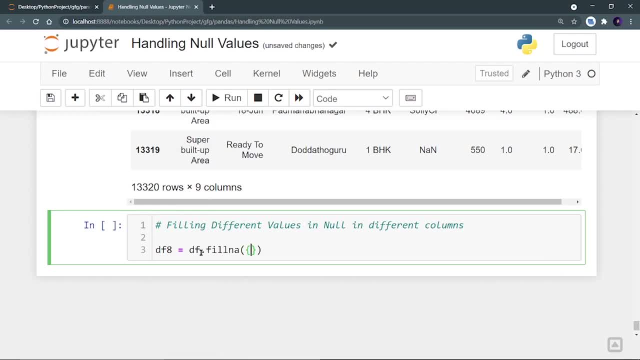 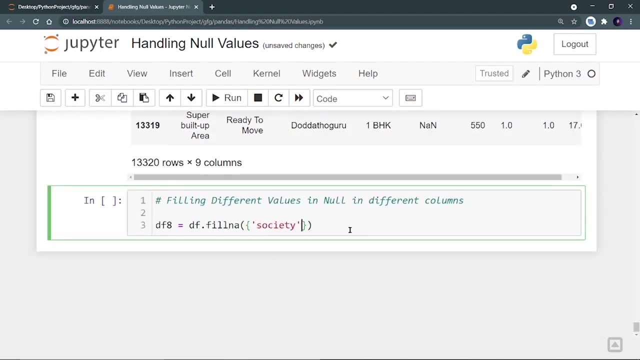 And over here you have to define a dictionary And inside this dictionary you have to define a key which will be your column name. So let's take the column name as society, And in society, you want to fill this with, let's say, abcd. right, 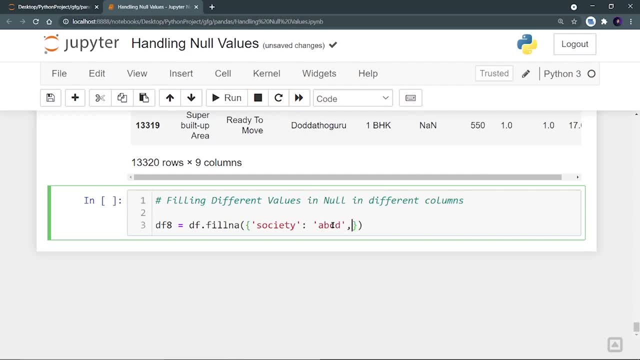 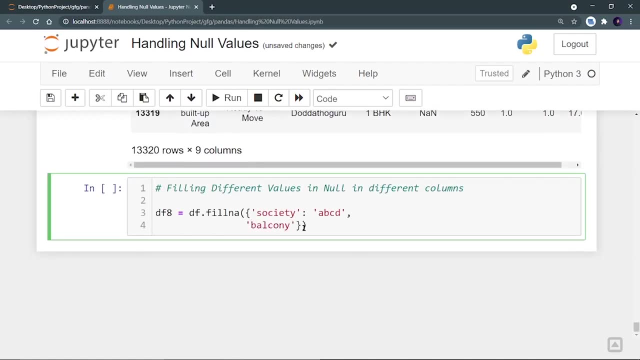 So let me put it in a string: abcd. And the second column name is balcony. So let's copy it and paste it. And here you want to fill the null value with def. And here you want to fill the null value with def. 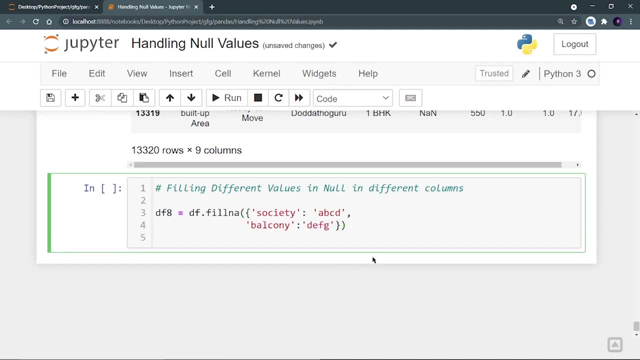 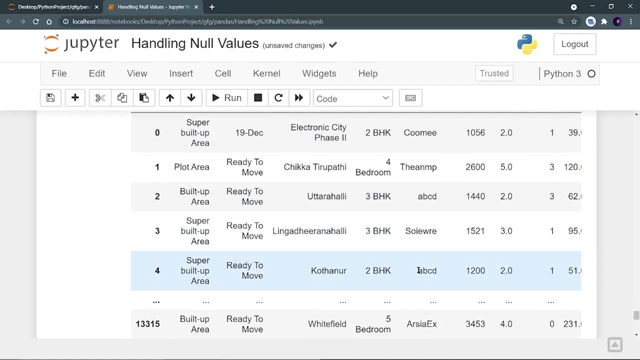 And here you want to fill the null value with def. And here you want to fill the null value with defg. right, Let's print df8 and let's see what we have got So over here I can see that in society my null value is filled with abcd and in balcony 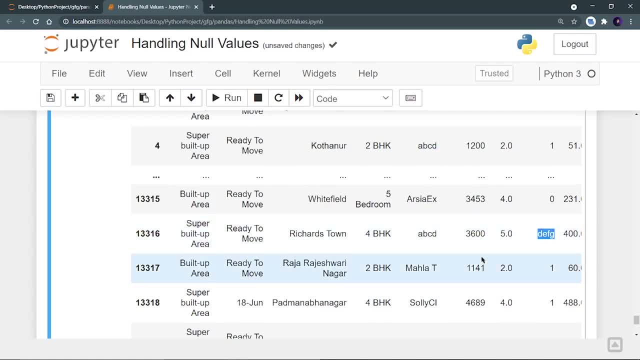 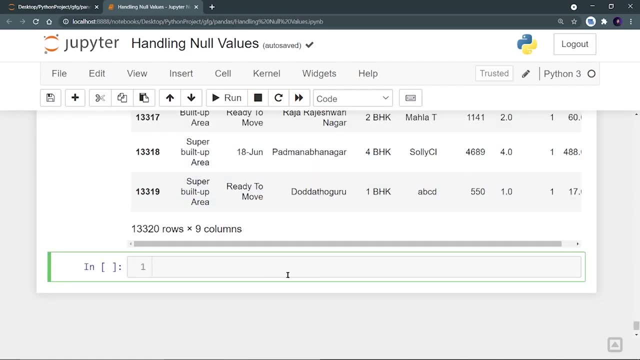 my null value is filled with defg. So here I can see that how I am filling the null values for different columns. right Now. let's see the next thing Now here, what I want to do is I want to fill the null value with the mean of the complete. 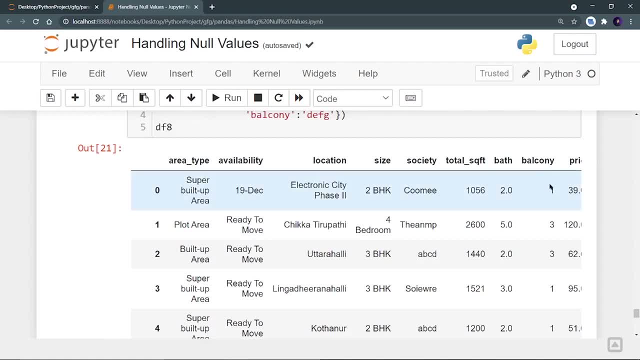 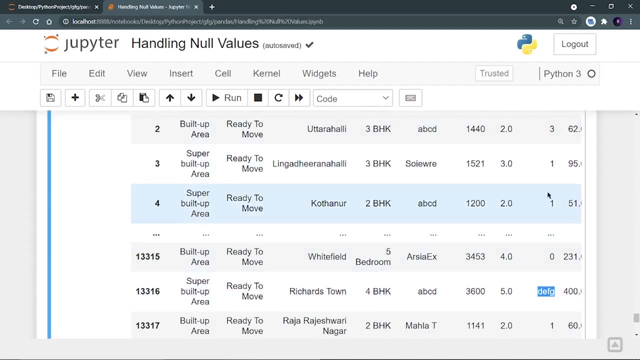 column right. So here I can see that This column is a numeric column right: 1, 3, 3, 1, 0, like this. So here I want that this null value should be filled with the mean of this complete numeric. 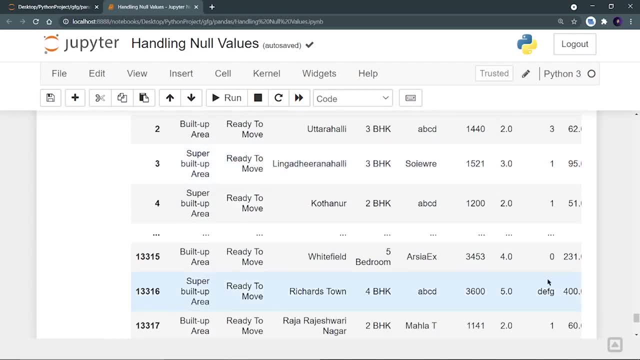 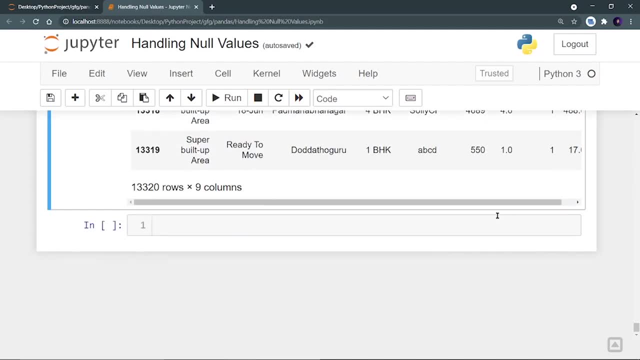 So here I can see that this column is a numeric column right: 1, 3, 3, 1, 0, like this. So here I want that this null value should be filled with the mean of this complete numeric column right. 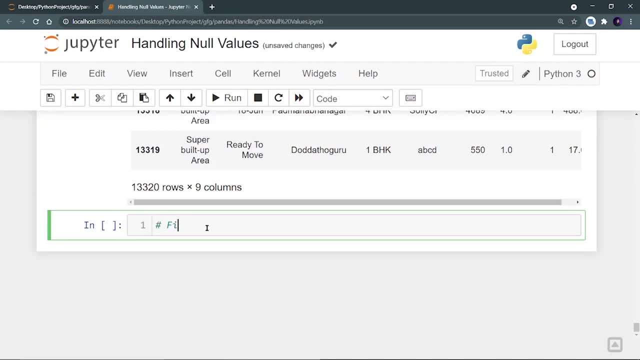 So here I let me put the topic filling null value with the mean of a column Right. So. So what I can do is I can create a new data frame. df9 is equal to dffillna and the value that is a parameter is going to be df add, and here you have to define the column name. 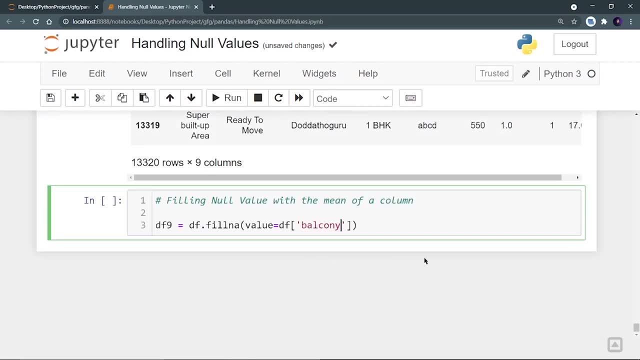 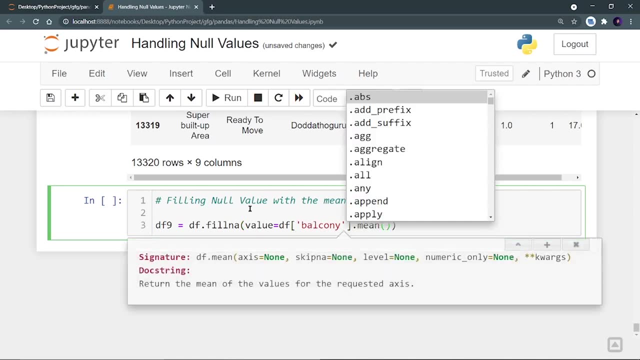 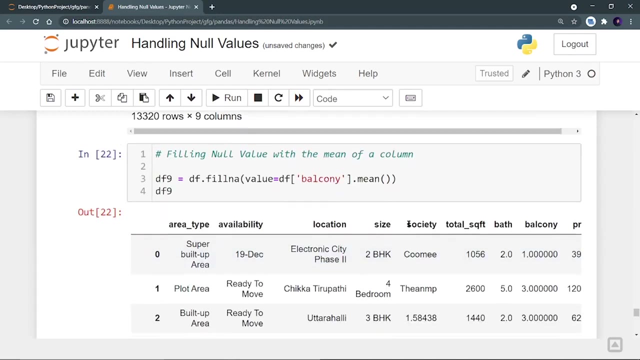 that is balcony. put it over here and you can just define dot mean. That means the mean value of this complete balcony column will be filled at the null places, right? So? So let me run it. So let's print df9,, let's run it, and I can see that in balcony, I can see that there. 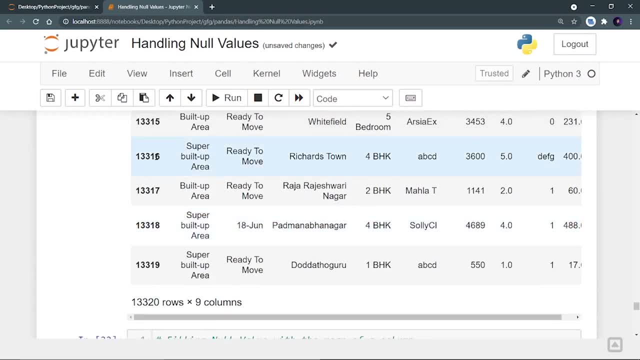 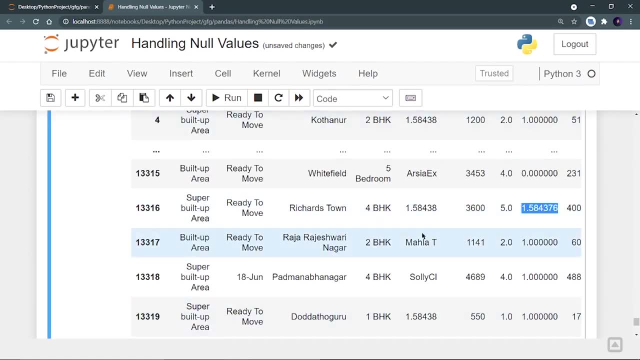 is no null value. Why? Because that null value, which is at position 1, 3,, 3, 1, 6, 1, 3,, 3,, 1, 6 is now filled with a mean of this complete column right. 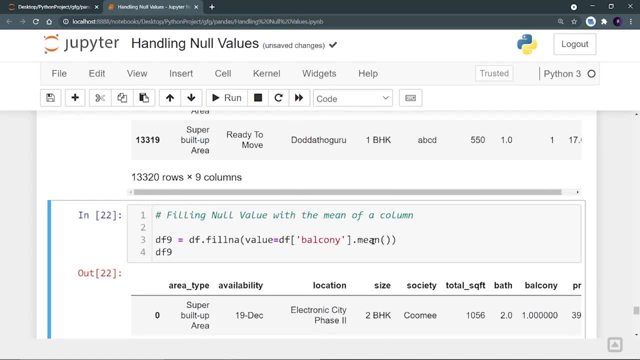 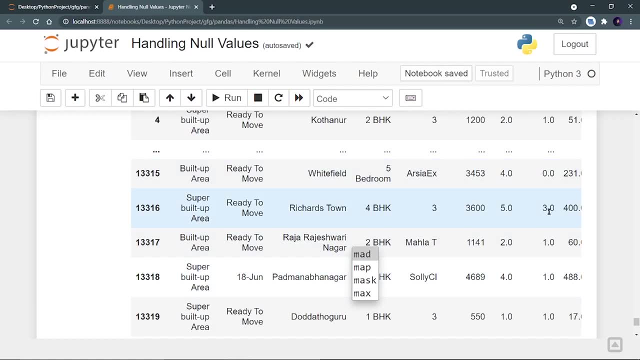 So it's totally up to you. You can also fill this with a max. So let's print it max over here and let's run it, And I can see that at 1, 3, 3,, 1, 6, it is now filled with the max of this complete column. 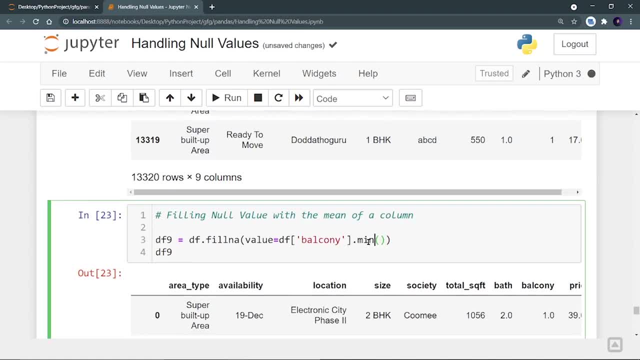 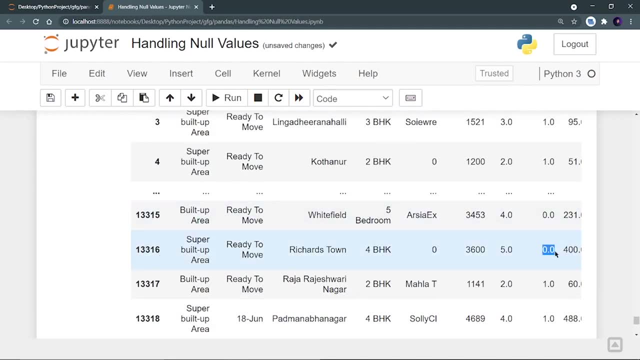 right, You can also fill it with a mean, So let's fill it with a min. That is, the minimum value will take the place of the null places. So here I can see that at 1,, 3,, 3,, 1, 6, it is zero, because zero is the minimum value. 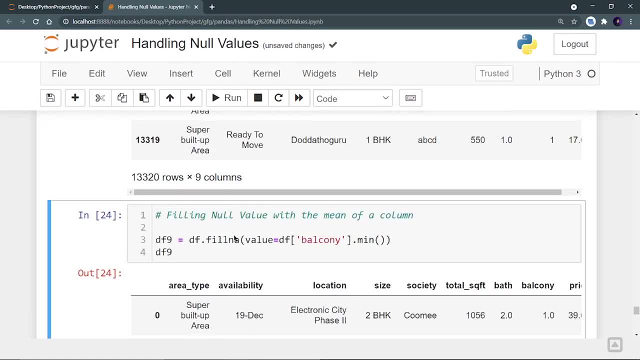 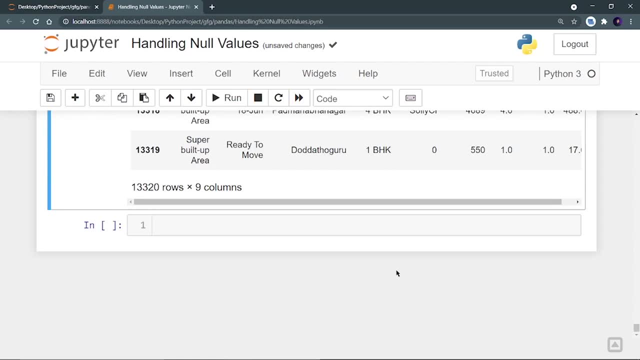 in this complete column. So we have seen the method fillna, that is, filling the null values. Now the next thing we are going to see is dropna. That is, we are completing the column. We are completely going to drop those rows, right. 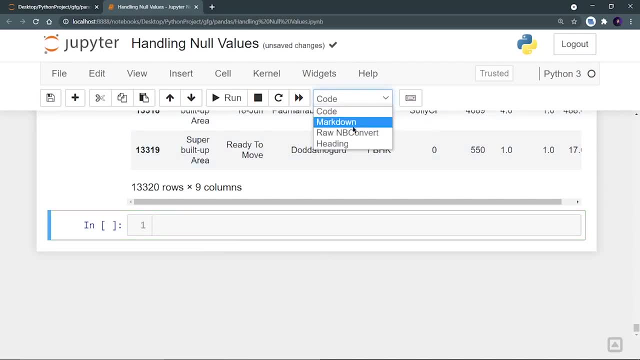 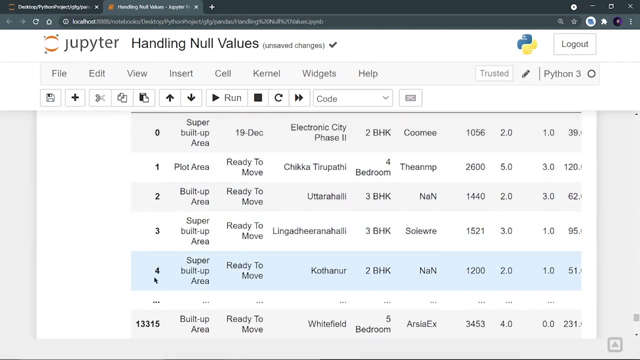 So what I can do is I can put a topic, So let me put a markdown dropna method right. So let's see first of all, the original data frame df, and I can see that this, that is, fourth index row, is having a null value. 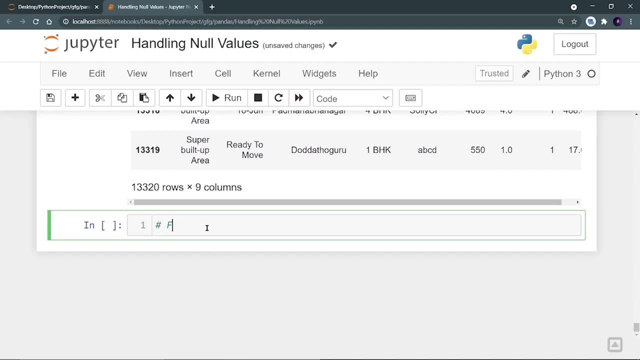 column right. So here I let me put the topic filling null value with the mean of a column right. So what I can do is I can create a new data frame. df9 is equal to df9.. df9 is equal to dffillna and the value that is a parameter is going to be df. add and here. 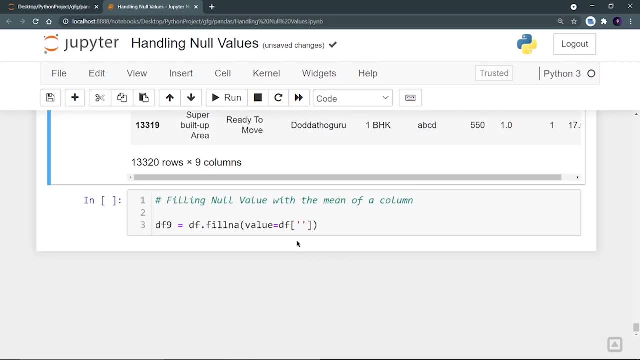 you have to define the column name. that is, balcony. put it over here and you can just define dot, mean. That means the mean value of this complete balcony column will be filled at the null places, right? So let me run it. So let's print df9. 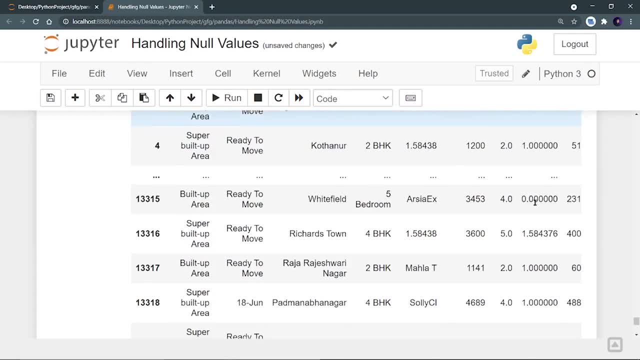 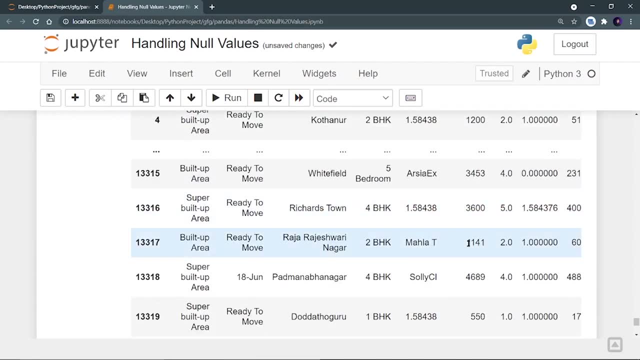 Let's run it. And I can see that in balcony. I can see that there is no null value. Why? Because that null value, which is at 1, 3, 3, 1, 6,, 1,, 3,, 3,, 1, 6, is now filled with. 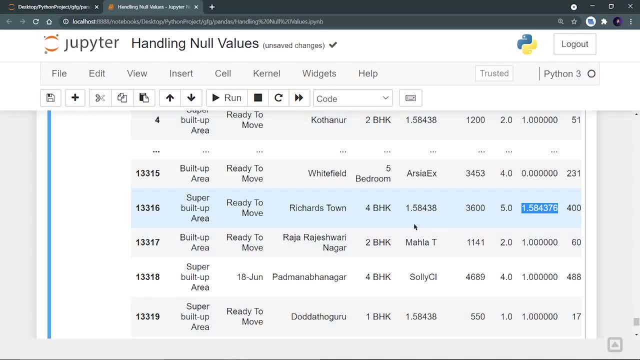 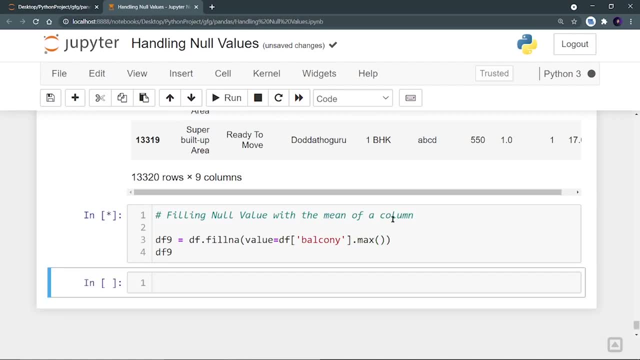 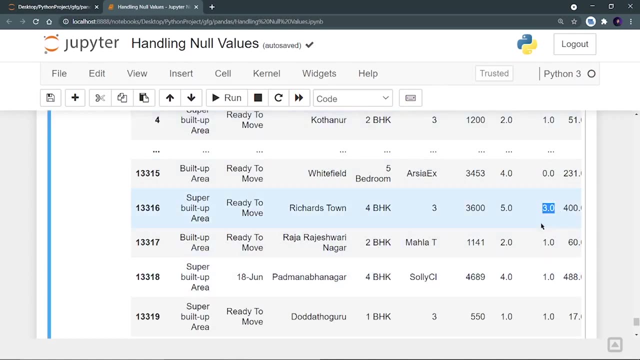 the mean of this complete column, right? So it's totally up to you. You can also fill this with the max. So let's print it max over here and let's run it, And I can see that at 1, 3, 3, 1, 6, it is now filled with the max of this complete column. 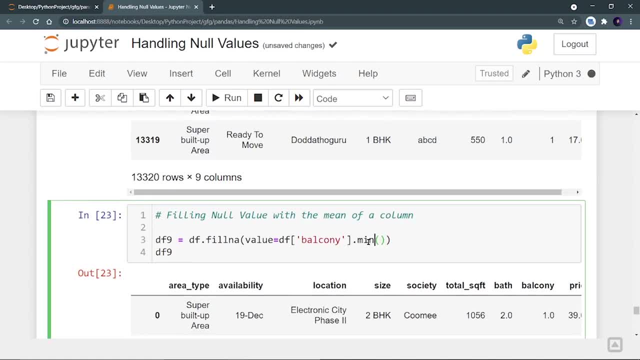 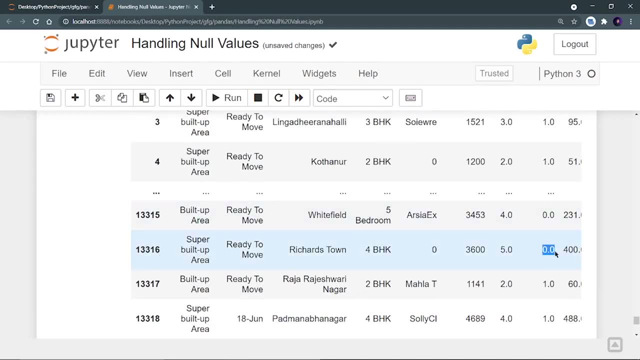 right, You can also fill it with a min, So let's fill it with a min. that is the minimum value will take the place of the null places. So here I can see that at 1,, 3,, 3,, 1, 6, it is zero. because zero. 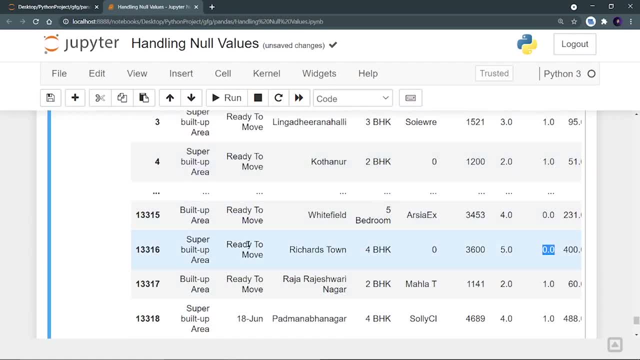 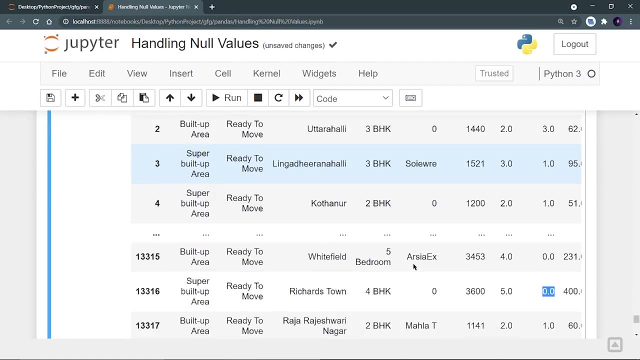 is the minimum value in this complete column. So we have seen the method fill any, that is, filling the null values. Now the next thing we are going to see is drop any, that is, we are completely going to drop those rows, right. So what I can do is I can put a topic. So 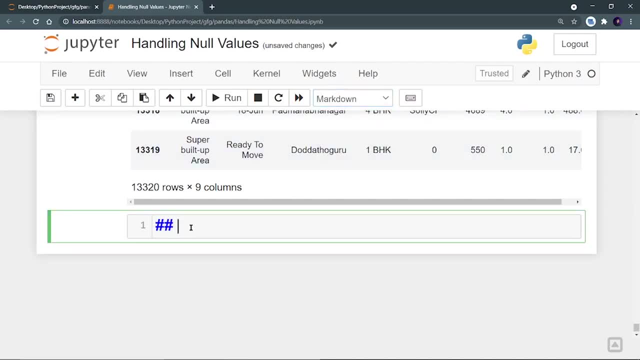 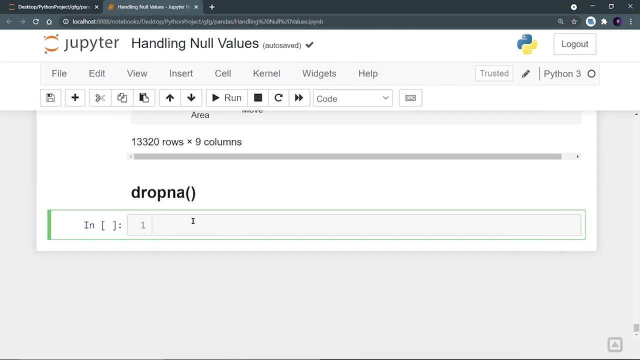 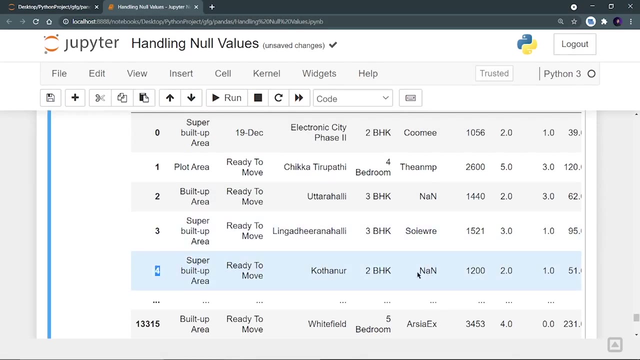 let me put a markdown. drop any method right. So let us see, first of all, the original data frame df, and I can see that this- that is fourth index row- is having a null value. Then I can see that the 1,, 3,, 3, 1, 6 row is having a null value and it is containing two. 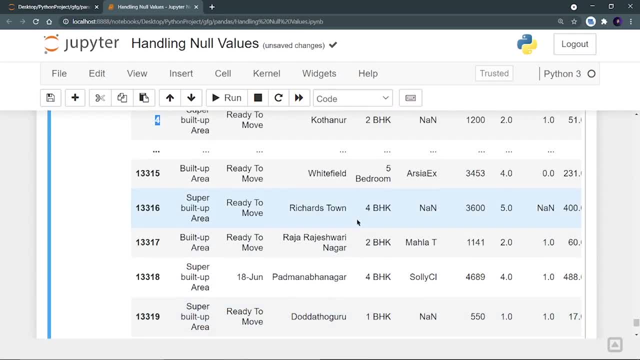 null values, by the way, and I can see it more, but there will be more null values also, right? So let me put a markdown. drop any method. So let me put a markdown- drop any method. So let me put a markdown. 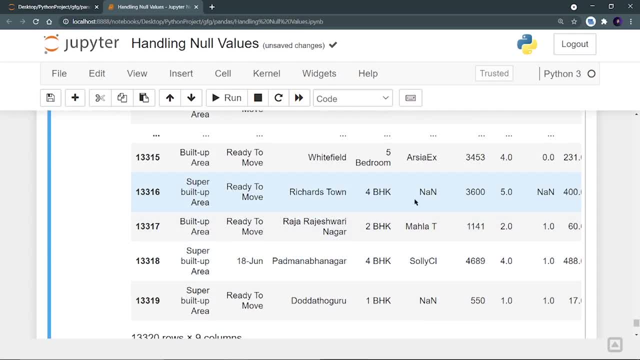 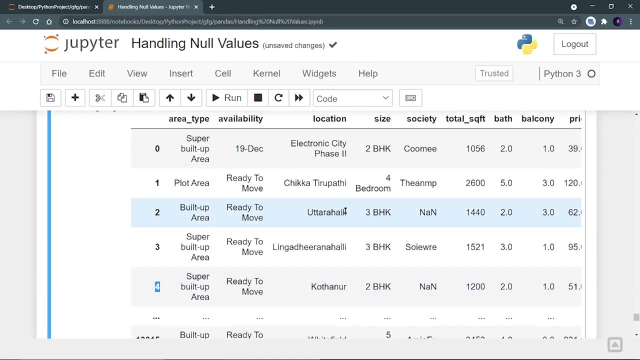 Then I can see that the 1,, 3,, 3, 1, 6 row is having a null value And it is containing two null values, By the way, and I can't see it more, but there will be more null values also, right. 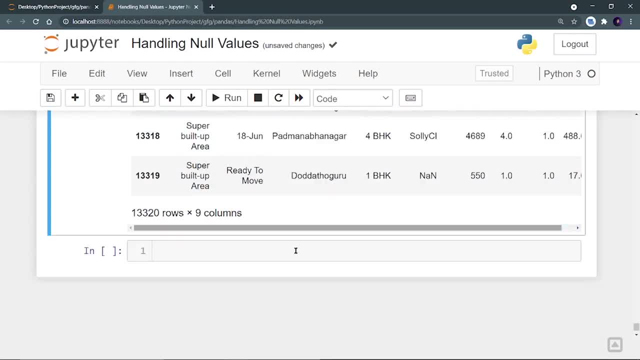 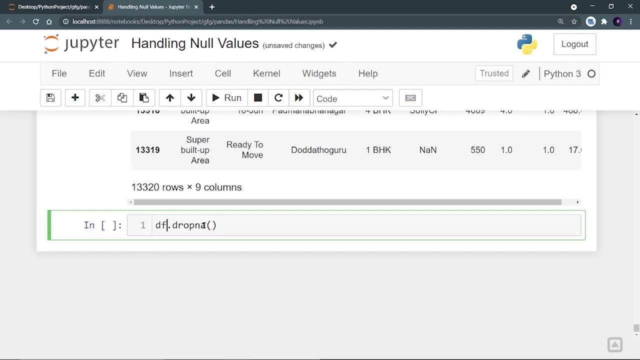 And I can see at index number two also, there is a null value right Now. if I'm going to run a function called dfdropna and let's dfdropna and let's save it in df10 and let's run it by printing df10, I can see that index number two, then four. 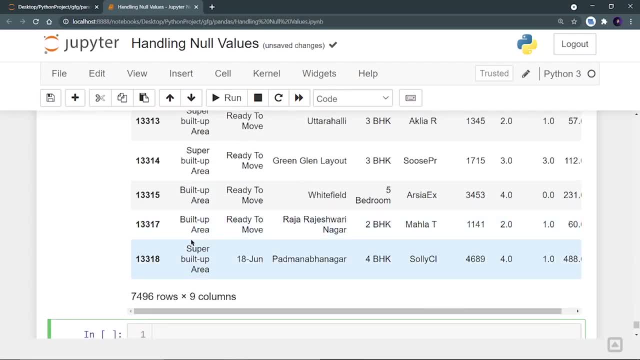 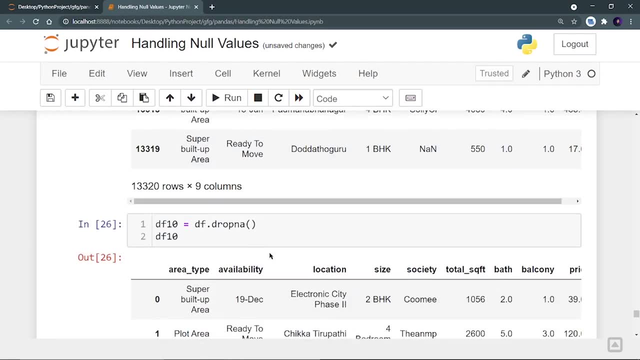 then 1, 3, 3, 1, 6.. And like this, Any row that is containing even one null value is removed from our data frame. So this simply drops those rows which contain even one null value, right. 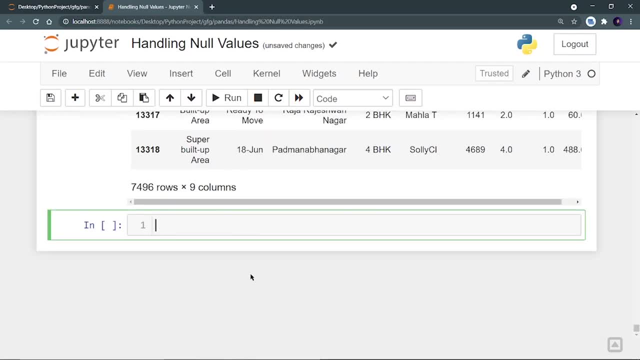 I hope you are understanding. Now, the second thing that comes in dropna is a parameter called how. right, So I'm going to do the same thing, that is, df11, dfdropna, but you have a parameter called how, and in this how parameter you can define multiple things. 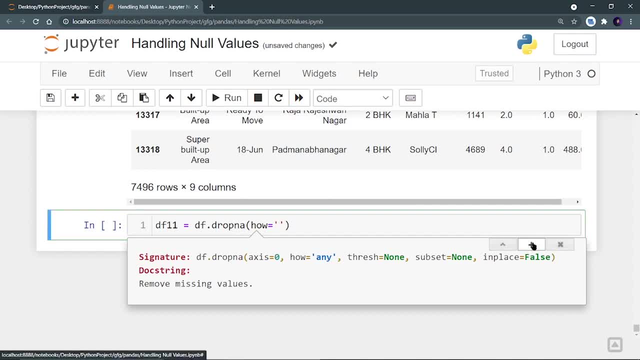 Let's see what we can define. So I'm clicking on shift plus tab and click on the plus icon And you can see in this how that we have values, two values we are we can fill. that is any and how. all right, 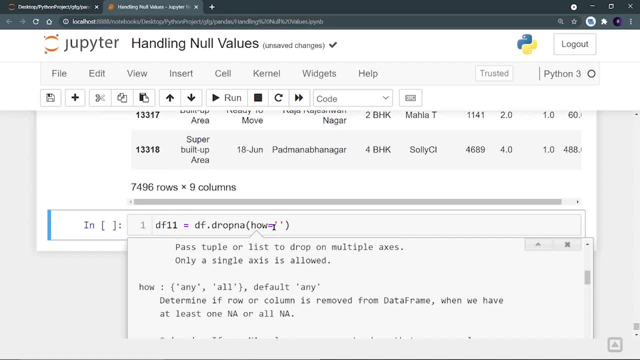 Any means if any of the cell in that row will be null, then that row will be removed or dropped. But all means if all the values in this complete row are null, that means null. null here, also, null here, also, null everywhere. null will be there in that row. 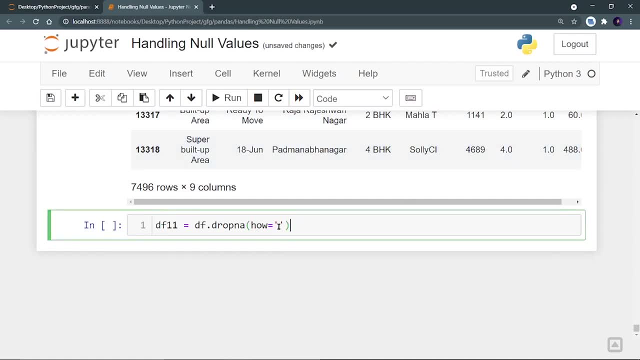 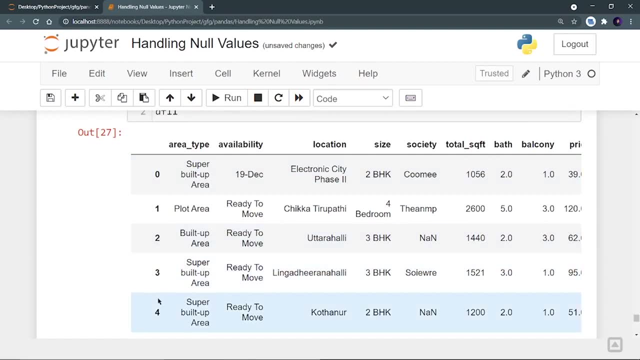 So then, then, and then only that row will be removed, otherwise it will not be removed. So let's print it all and let's print df11.. I can see that index number two and four are still there because they don't contain all. 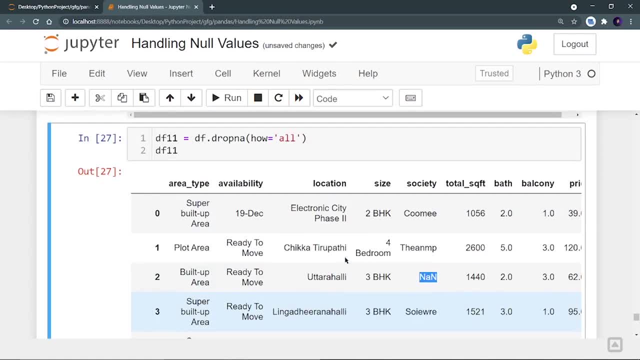 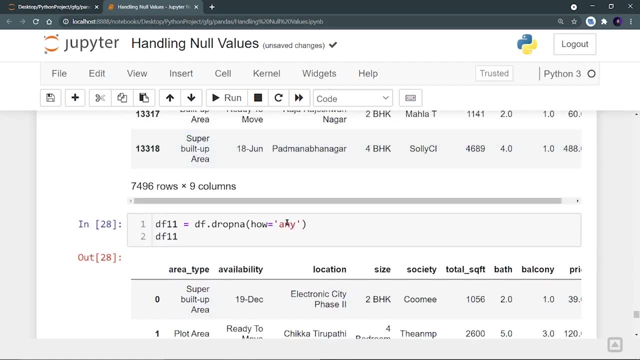 the values null. They contain only one value, null right- And if I print it any, I can see that two and four are not there. why? Because they contain at least one null value, any null value right. So this was how we drop the null values. 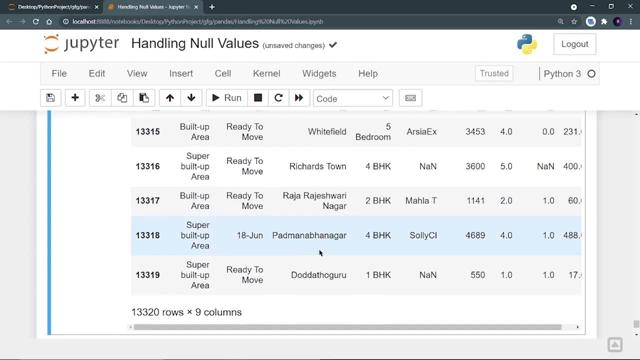 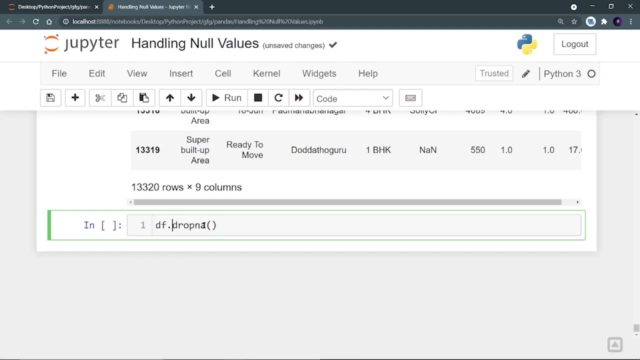 And I can see at index number two also, there is a null value right Now. if I'm going to run a function called dfdropna and let's dfdropna and let's save it in df10, and let's run it by printing df10,, I can see that index number two. then 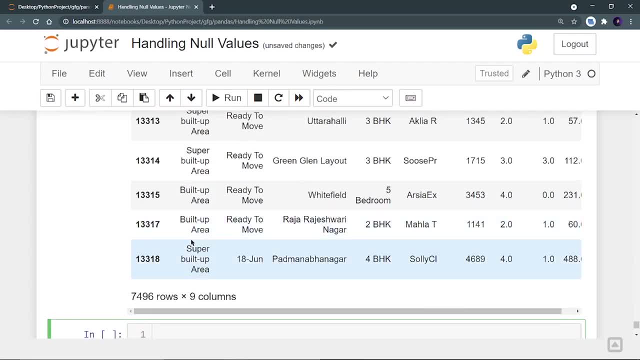 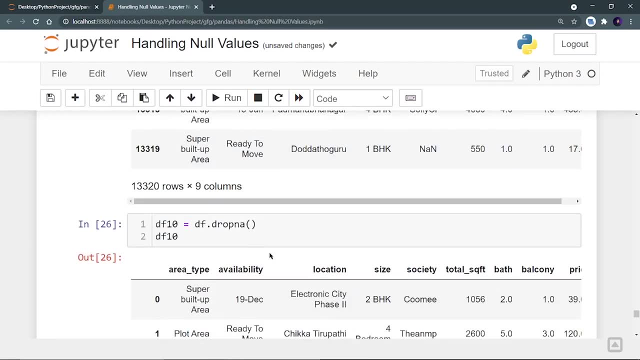 four, then one three, three, one six, and like this, any row that is containing even one null value is removed from our data frame. So this simply drops those rows which contain even one null value. right? I hope you are understanding. 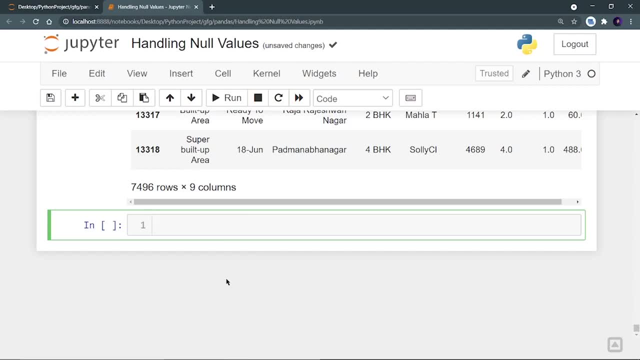 Now the second thing that comes in dropna is a parameter called how. right, So I'm going to do the same thing, that is, df11, dfdropna, but you have a parameter called how, and in this how parameter you can define multiple things. 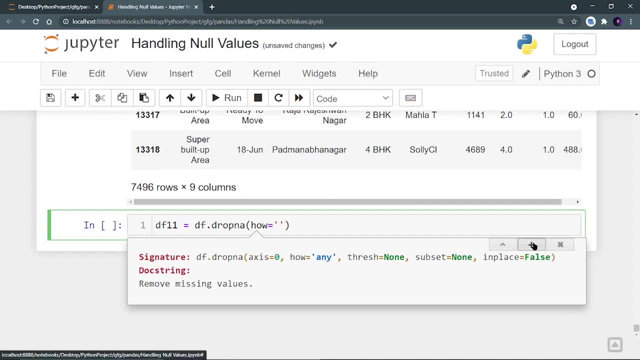 Let's see what we can define. So I'm clicking on shift plus tab and click on the plus icon and you can see in this how that we have values, two values we can fill. that is any and how. all right. 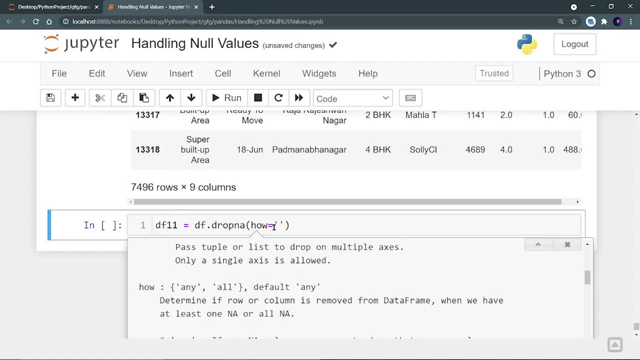 Any means if any of the cell in that row will be null, then that row will be removed or dropped. but all means, if all the values in this complete row are null, that means null. null here, also, null here, also, null everywhere. null will be there in that row then and then. 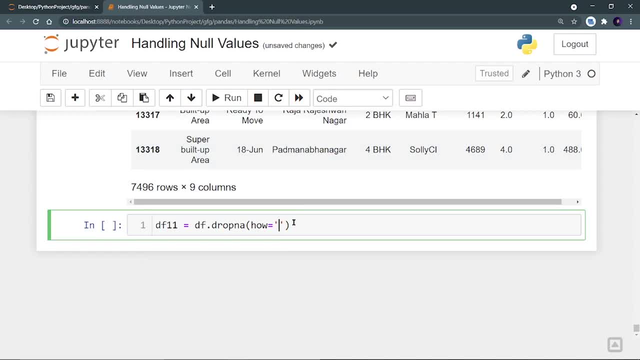 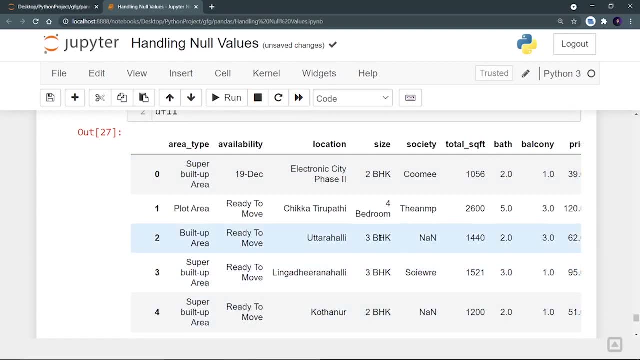 only that row will be removed, otherwise it will not be removed. So let's print it all And let's print df11,. I can see that index number 2 and 4 are still there because they don't contain all the values null. they contain only one value: null, right. 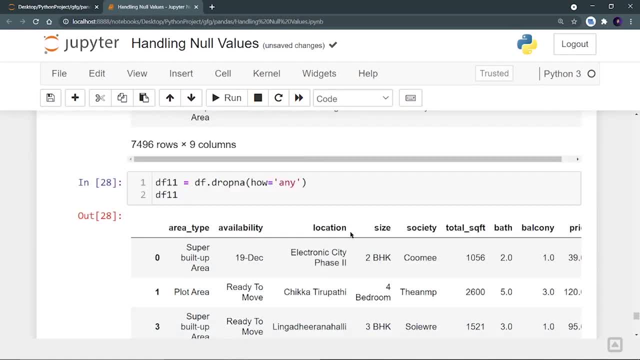 And if I print it any, I can see that 2 and 4 are not there. why? Because they contain at least one null value, any null value, right? So this was how we drop the null values using the dfdropna function. 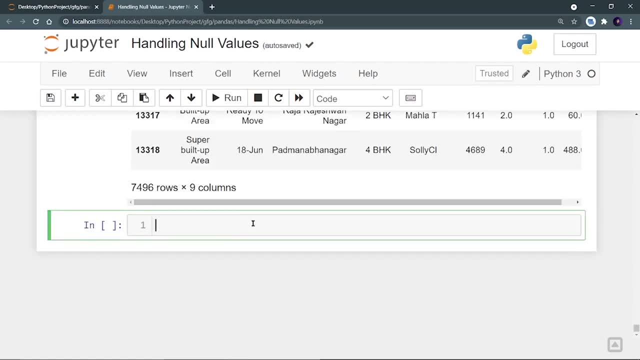 Now the third function that we are going to see in this video is dfdropna. So we are going to see that dfdropna. So we have the function name dfreplace, right? So let me put the markdown and the function name is replace. 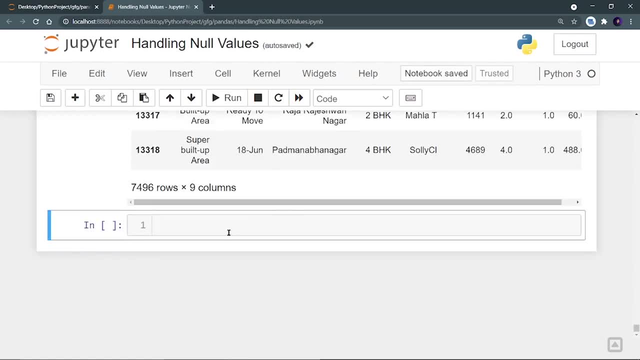 Using the dfdropna function. Now, the third function that we are going to see in this video is dfreplace, right? So let me put the markdown and the function name is replace. So here, as the name is suggesting, we have to replace the null values, right? 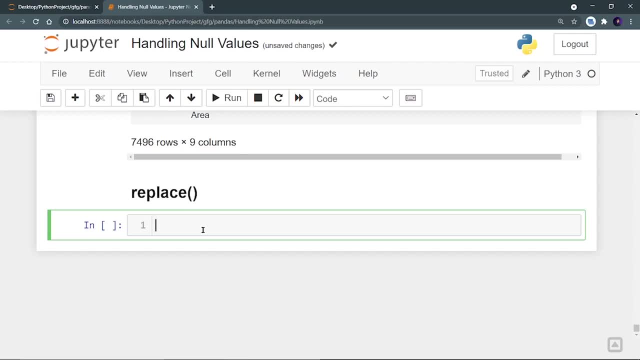 It is almost similar to fillna, but here we get some extra functions. So let's see what we can do. So we have to create another data frame called dfdropna. So dfnulldft12 is equal to dfreplace And we have a parameter- first parameter, called to replace. 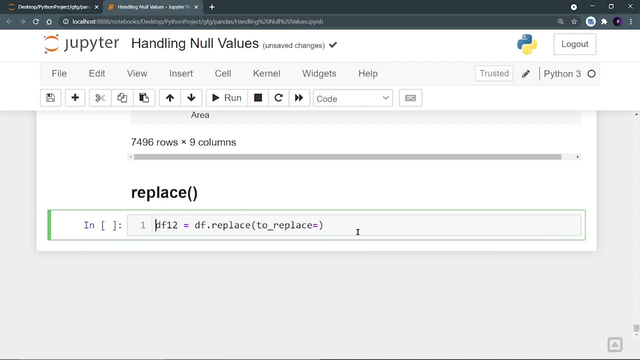 That means what we want to replace. So here we have to import numpy, because I can't write none like this null, like this right. So we have to import numpy as np, because numpy contains an object for null values, and here we can write npnn, right. 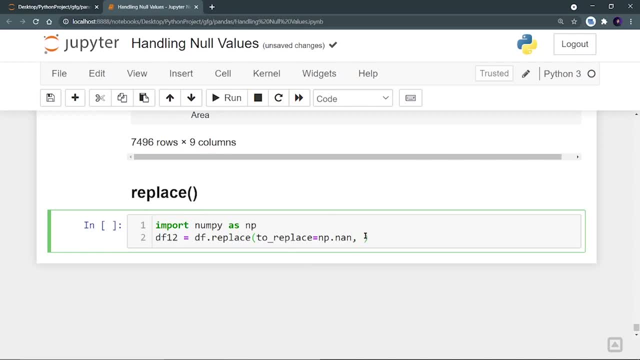 So we want to replace the null values. and here you have to define which value you want to replace with the null values, right? So here I have to write: value is equal to. let's print it this number. So wherever the null value will be there, it will be replaced by this number. right? So let's print the f12. and here I can see: 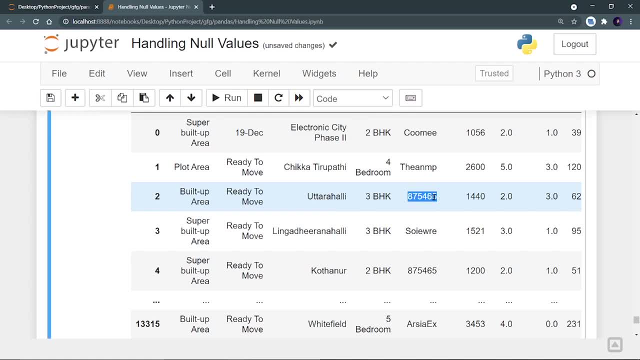 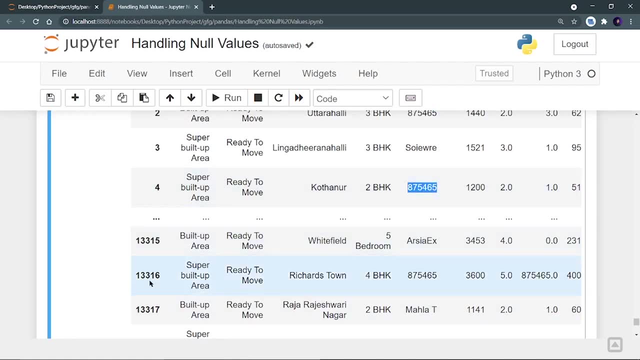 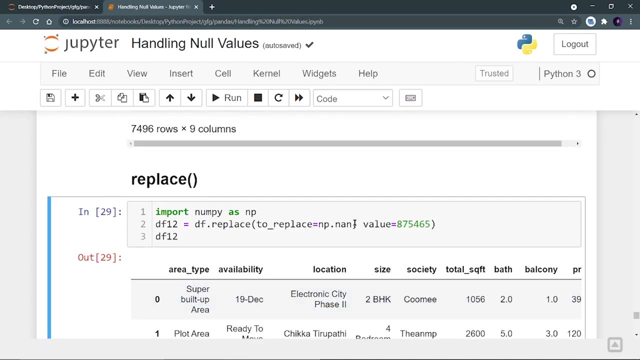 that index number 2, it was containing a null value, but now it is containing this number. and at index number 4, it was containing a null value, but now it is this number. Here also, 13316, it was having a null value, but now it is containing this number, right. So this function has replaced all. 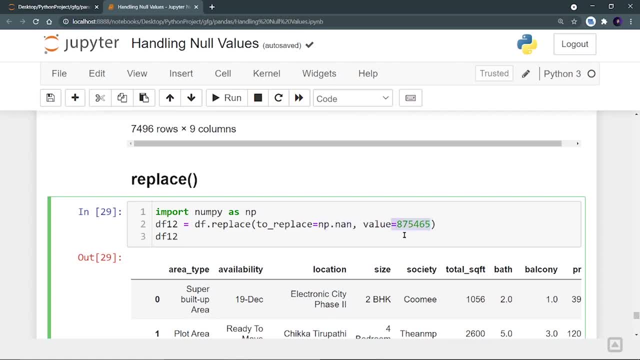 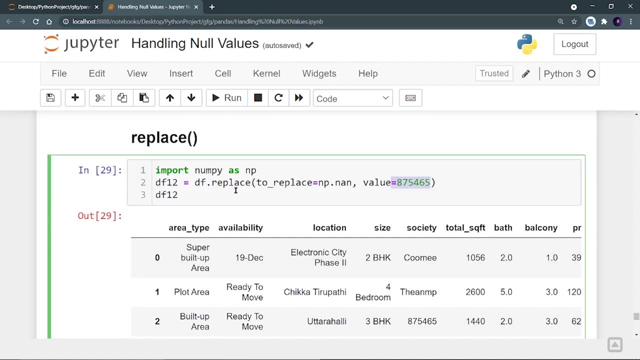 the null values with this number and you can put anything right. you can put any number, it will replace the null values. and using this replace function, you can not only fill the null values. you can not only replace the null values, but you can also replace any value. Let's say, I want to. 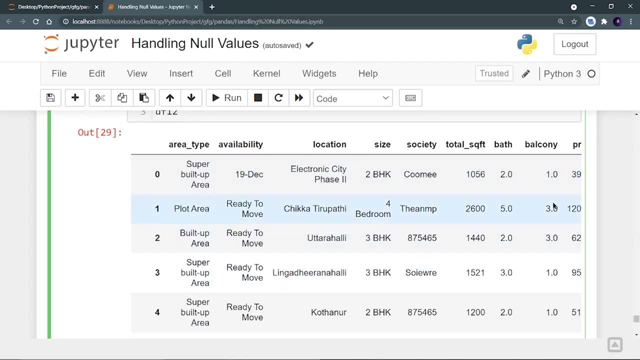 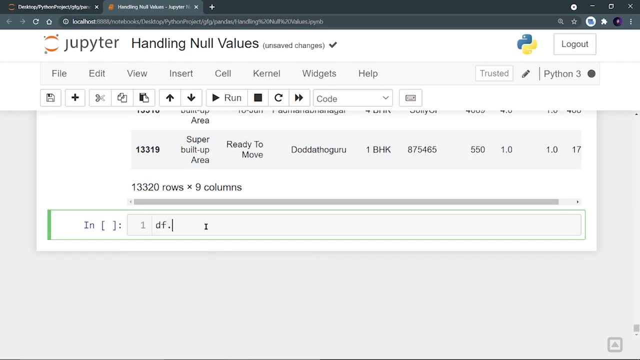 replace 3.. So here I can see that balcony is containing a lots of things. So wherever I am getting 3, I want to replace them with 5.. So let's do it So: df dot replace. to replace 3 float number with a. 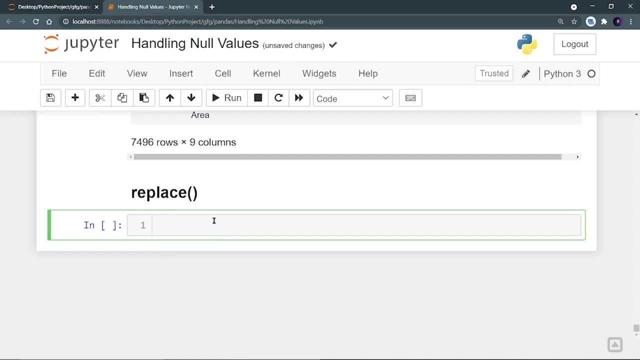 So here, as the name is suggesting, we have to replace the null values. right, It is almost similar to fill name, but here we get some extra functions. So let's see what we can do. So we have to create another data frame called df12 is equal to dfreplace. 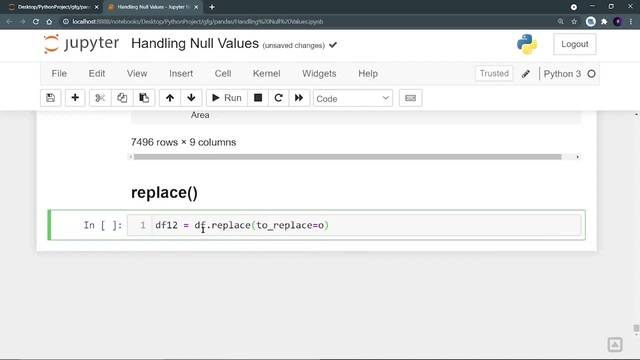 And we have a parameter, first parameter called toReplace. that means what we want to replace. So here we have to import numpy, because I can't write none like this null, like this right. So we have to import numpy as np, because numpy contains an object for null values. And here 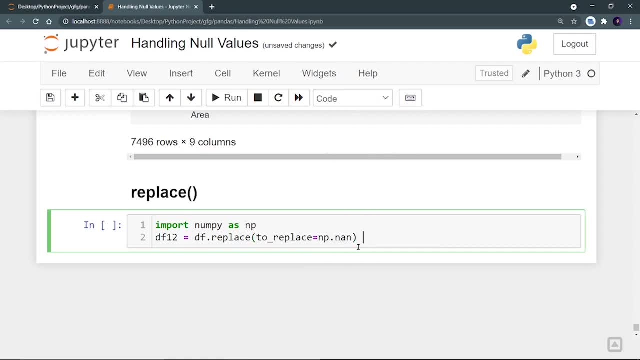 we can write npnn, right? So we want to replace the null values. and here you have to define which value you want to replace with the null values, right? So here I have to write: value is equal to- let's print it, this number, So wherever the null value will be there. 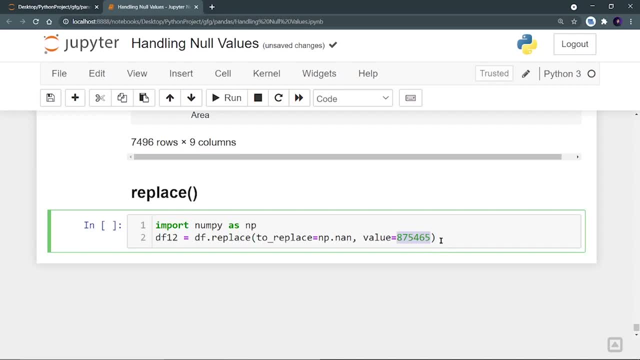 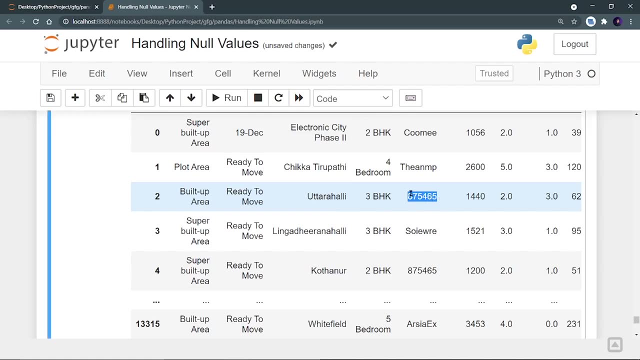 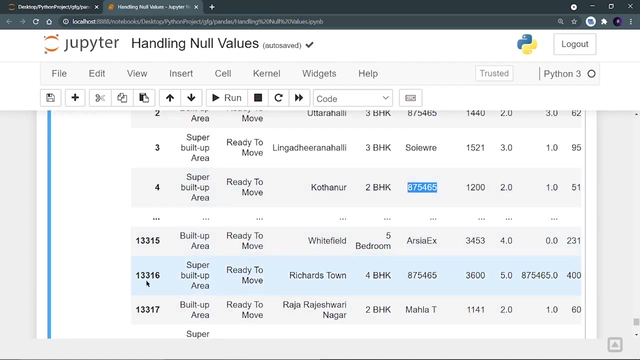 it will be replaced by this number, right? So let's print df12.. And here I can see that index number 2, it was containing a null value, but now it is containing this number. And at index number 4, it was containing a null value, but now it is this number. Here also, 13316,. 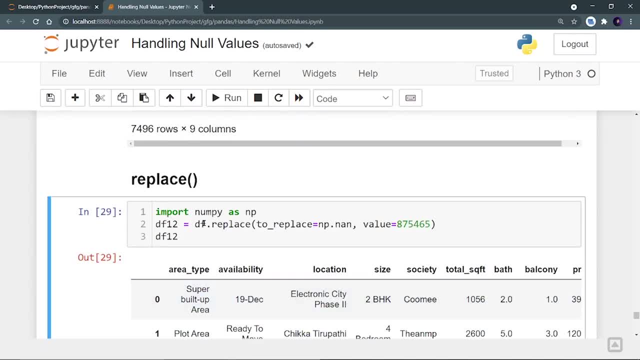 it was containing a null value, but now it is this number. And at index number 4, was having a null value, but now it is containing this number right. So this function has replaced all the null values with this number and you can put anything right. You can put any number. 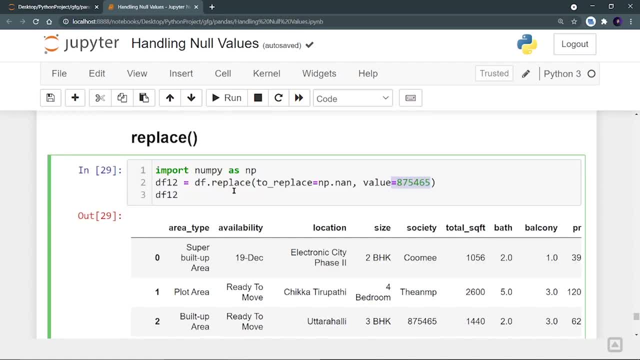 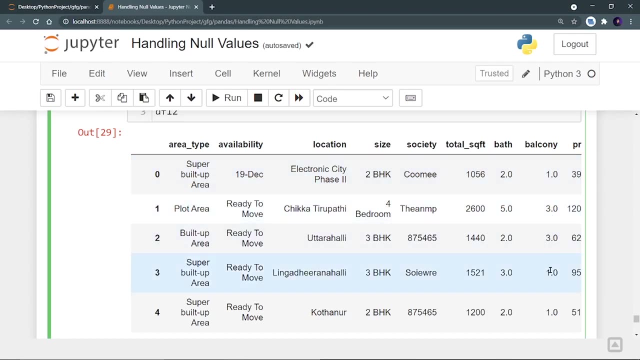 it will replace the null values. And using this replace function, you can not only fill the null values, you can not only replace the null values, but you can also replace any value. Let's say, I want to replace 3.. So here I can see that balcony is containing a lot of things. 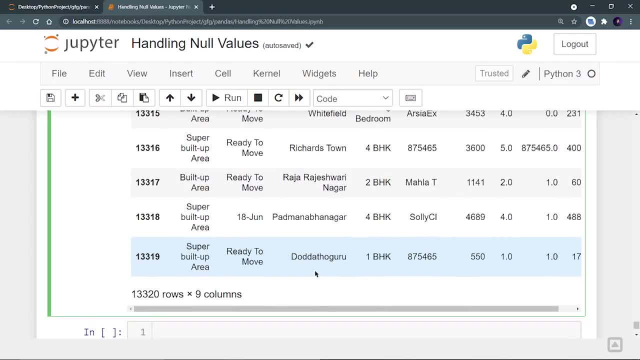 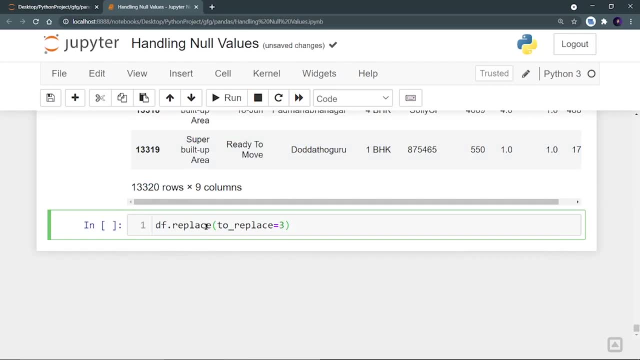 So wherever I am getting 3, I want to replace them with 5.. So let us do it So: def dot replace to replace 3 float number with a value 5.0,. right, Let us create another data frame: df. 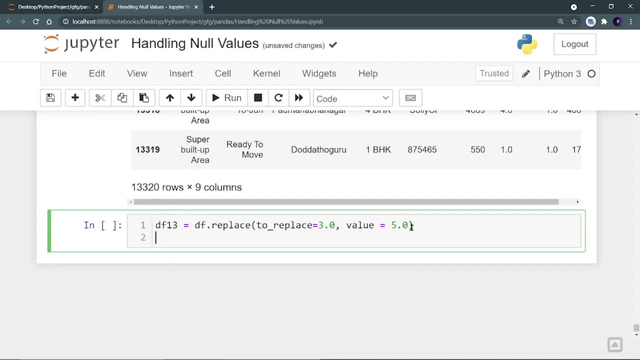 13 is equal to, and let us print it. So this is the beauty of the replace function: that it is not restricted to the null values. We can replace any value with another value, So let us print it. And I can see that wherever 3 was there, now it is 5, right. So this is the beauty of the 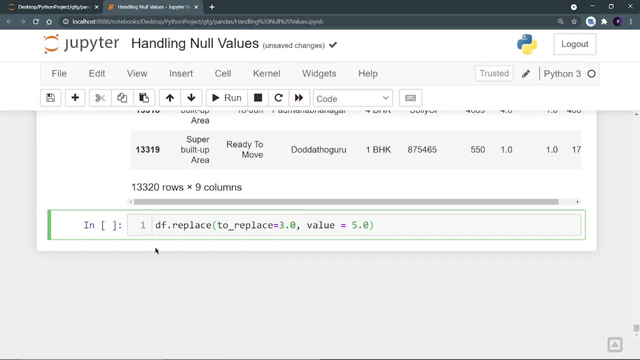 value 5.0. right, Let's create another data frame. df 13 is equal and let's print it. So this is the beauty of the replace function, So let's print it. So this is the beauty of the replace function: That it is not restricted to the null values. We can replace any value with another value, So let's. 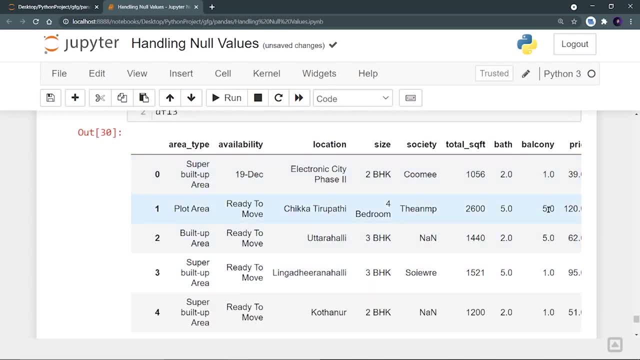 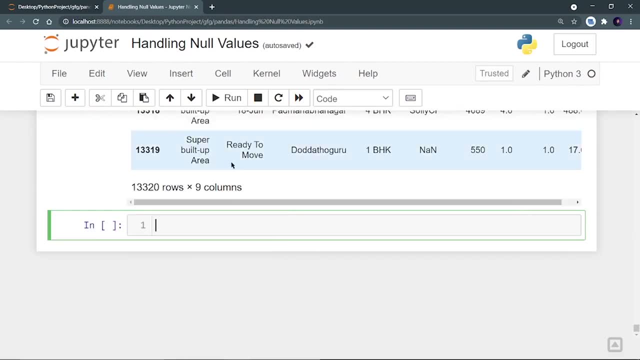 print it and I can see that wherever 3 was there, now it is 5 right. So this is the beauty of the replace function. Now, the last method that we are going to see to fill the null values is df, dot interpolate. So let's put the topic interpolate. So, as the name suggests, it uses different methods. 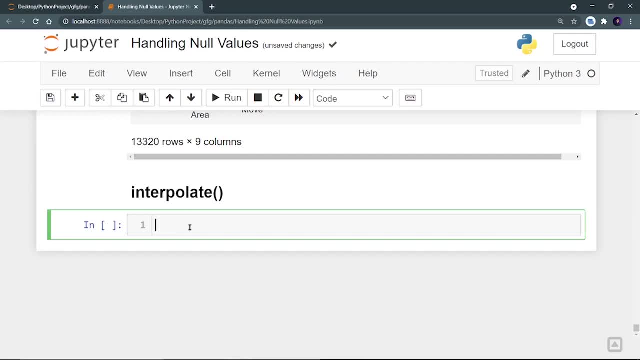 to interpolate the values. It interprets the values right. So let's say, my data frame is containing a column with the values like 1 then 2, then 3 then 4, and I can see that. I can see that it is having a null value like this and it is having 6 over here. it is having 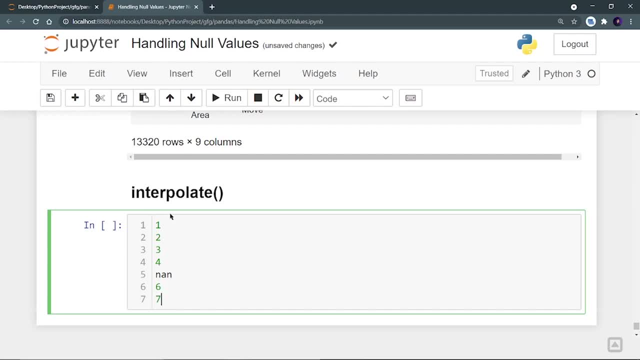 7 over here. So this is a very basic example and this interpolate function is going to interpret these values and it is going to fill this value automatically by 5, right, And there are various methods in this interpolate. So as, first of all, the method is linear, So it is going to consider: 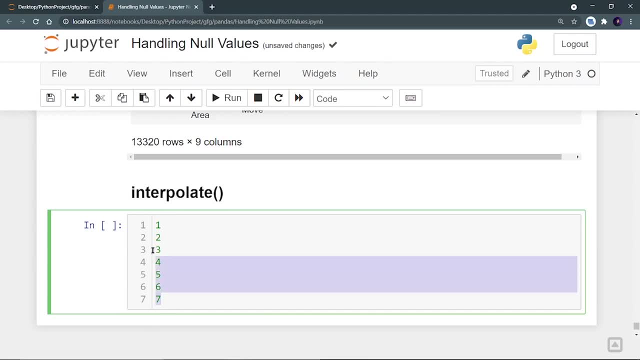 those values as a null value. So let's say my data frame is containing a column with a value of 5, then I can see that it has linearly distributed as we saw in this example. Let's say- I took one more example- as 5. then let's say it is having null value and it is having 6.. Null value and it is. 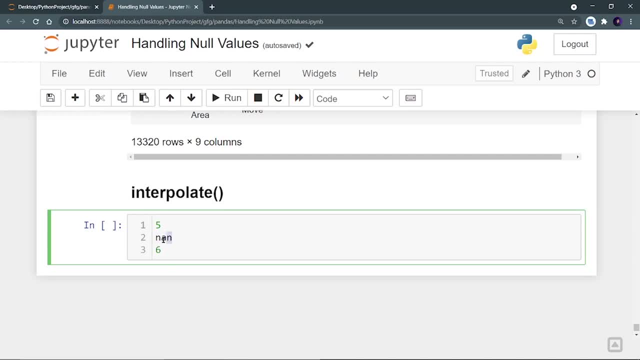 having 6 over here. So this interpolate function is going to interpret these values, all these values, and it is going to fill the nn value with the mean of these two values, So it will be 5.5.. So like this, it is a very useful function for filling the null values. Now let's use this. 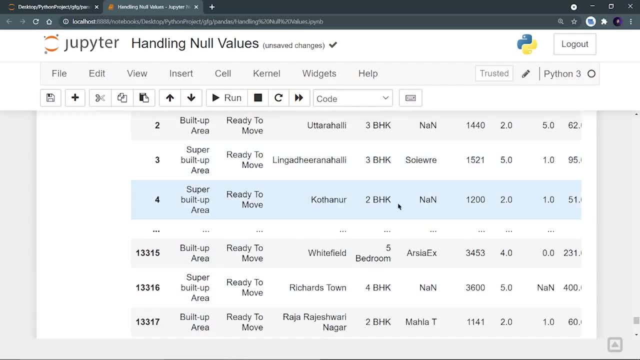 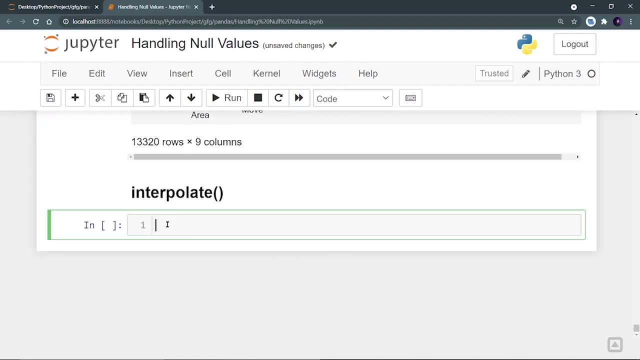 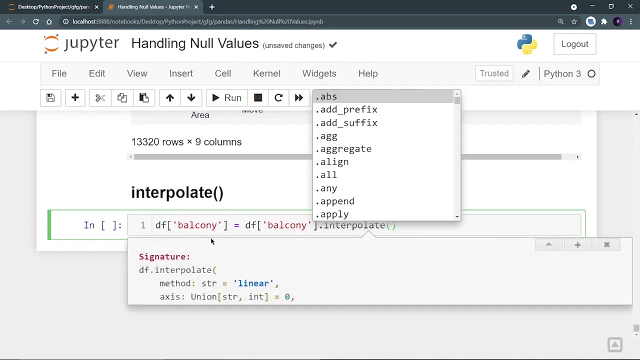 one, and we will use the linear method for filling the null values in balcony column, right. So let's do it So. as we are working on this balcony column, I am going to call only the balcony column, So df at balcony will be df at balcony, dot interpolate. Then you have to define a method. 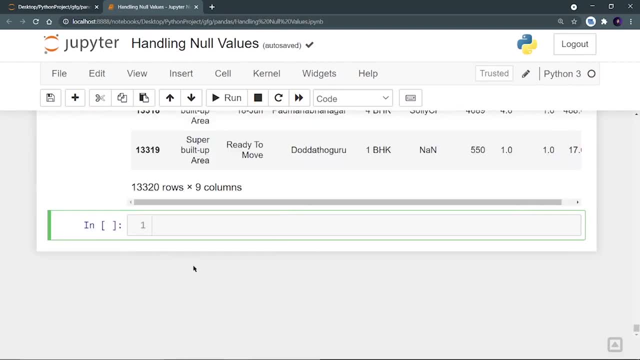 replace function. Now, the last method that we are going to see to fill the null values is dfinterpolate, So let's put the topic interpolate. So, as the name suggests, it uses different methods to interpolate the values. It interprets the values right, So 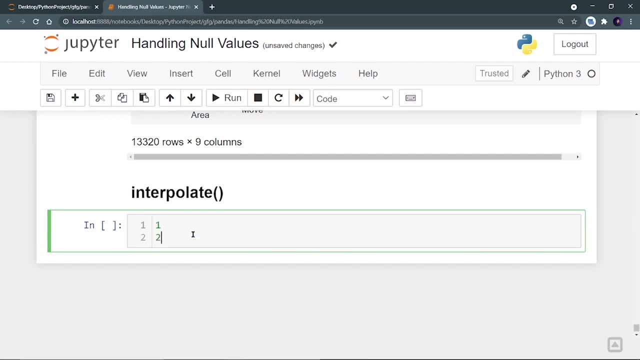 let's say, my data frame is containing a column with a values like 1, then 2, then 3, then 4.. And I can see that. I can see that it is having a null value like this And it is having 6 over here. 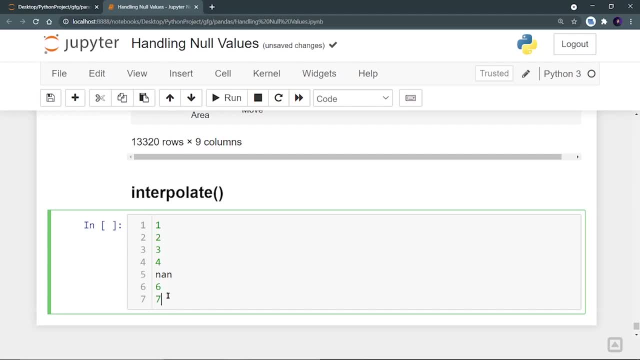 it is having 7.. So this is a very basic example And this interpolate function is going to interprete these values and it is going to fill this value automatically by 5.. And there are various methods in this interpolate. So first of all, the method is linear, So it is. 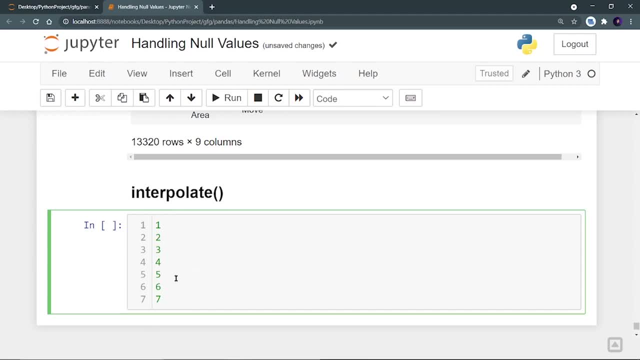 going to consider those values as linear values, because these values are 2'd or so many right linearly distributed, as we saw in this example. Let's say- I took one more example- as 5, then let's say it is having null value and it is having 6. Null value and it is having 6 over here. So 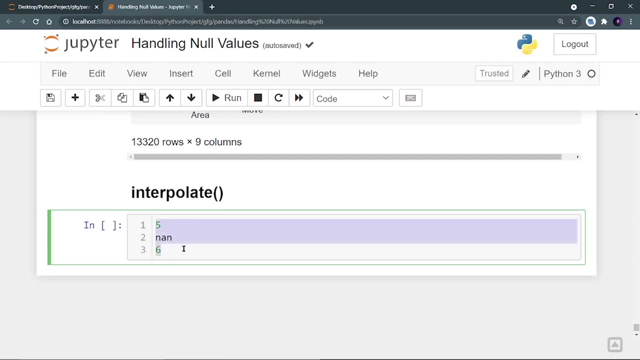 this interpolate function is going to interpret these values, all these values, and it is going to fill the nn value with the mean of these two values, So it will be 5.5.. So, like this, it is a very useful function for filling the null values. Now let's use this function and 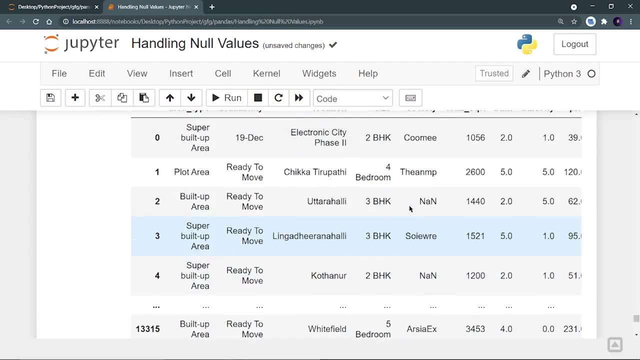 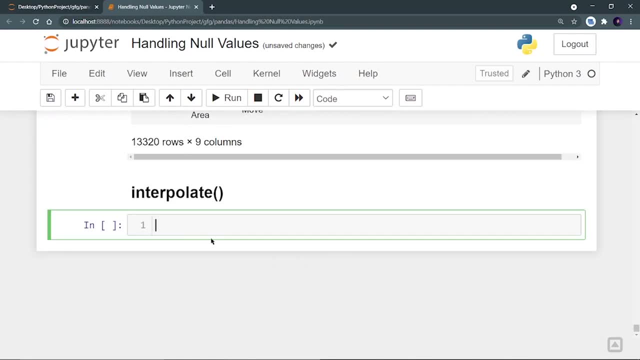 we will use a linear method for filling the null values in balcony column, right? So let's do it So. as we are working on this balcony column, I am going to call only the balcony column, So df at balcony will be df at balcony dot interpolate. 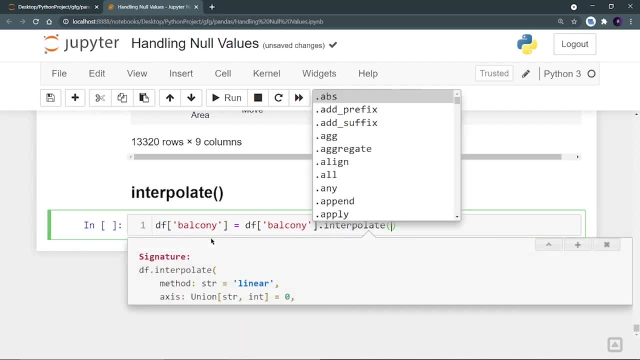 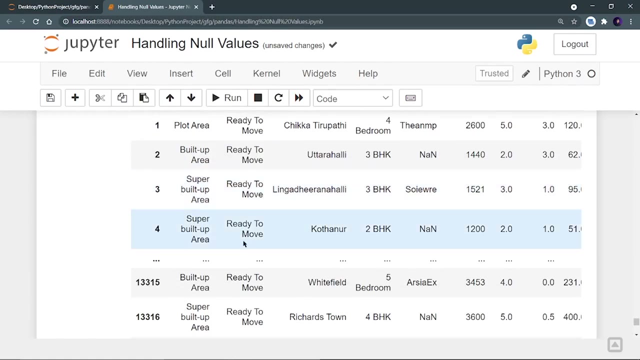 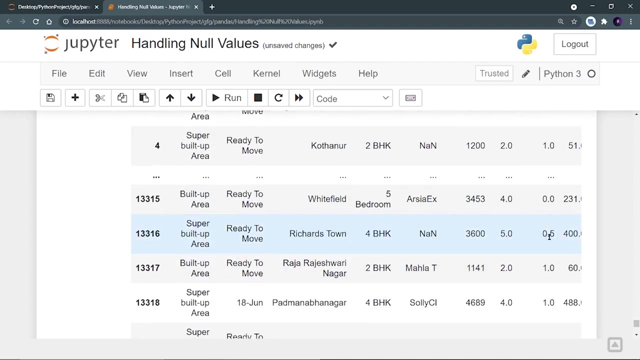 and then you have to define a method, and my method will be linear and let's try to run it. So let's print df and we can see that there was a null value at index 13316, and now, if I see 13316,, 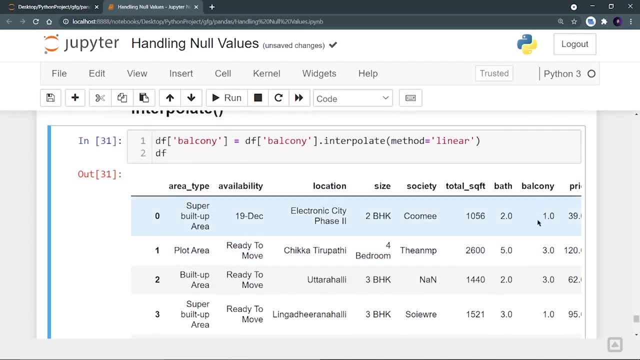 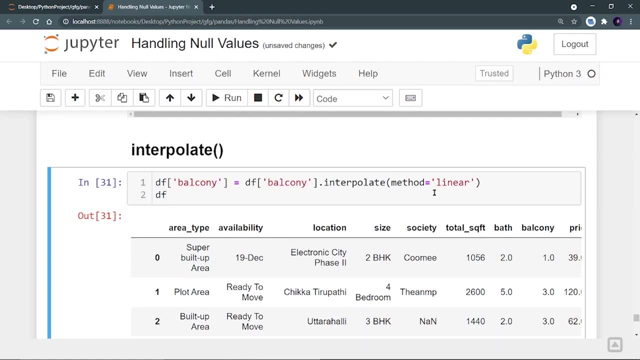 it has filled, or it has interpolated, this complete column, and it has filled it with 0.5, right? So this is how this interpolate function works. Now you have some more parameters in this, So let's see one more parameter, that is: